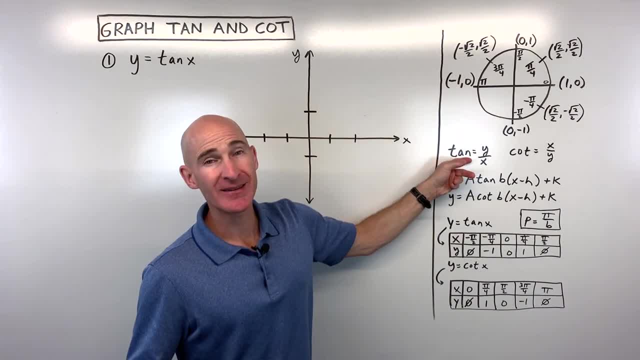 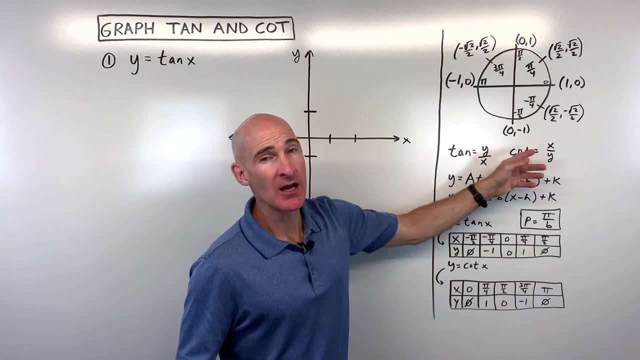 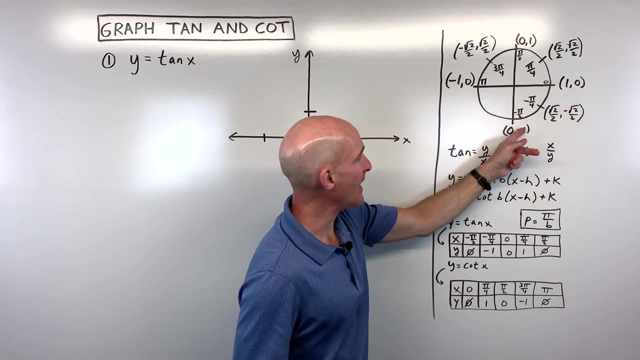 previously Remember. on the unit circle, when you calculate the tangent, it's the y-coordinate divided by the x-coordinate, whereas the cotangent is the x divided by the y. So let's start off by graphing just your basic tangent graph using the unit circle. So if we start over here at negative pi, 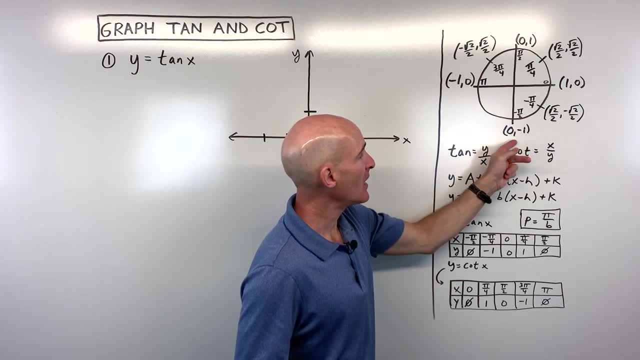 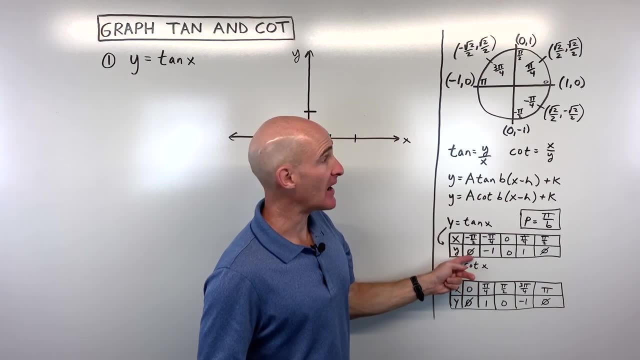 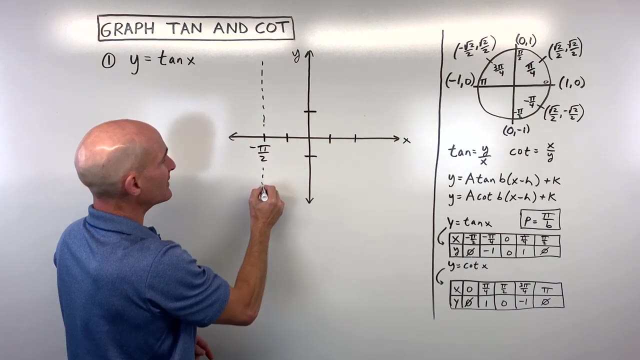 over 2, remember negative. you're going clockwise and the tangent would be negative, 1 divided by 0, which you can't do. So you can see that's going to be undefined and we're going to get a vertical asymptote. So let's just put here negative pi over 2 and draw that dashed or dotted line, that asymptote. 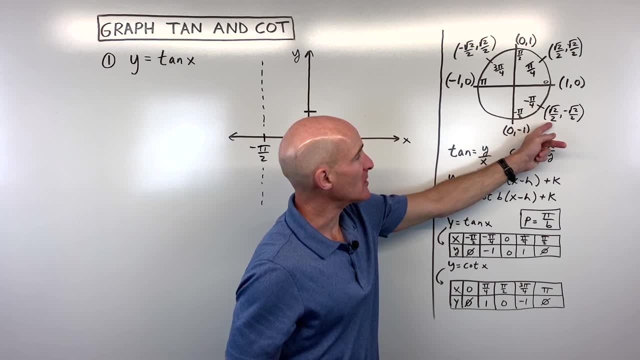 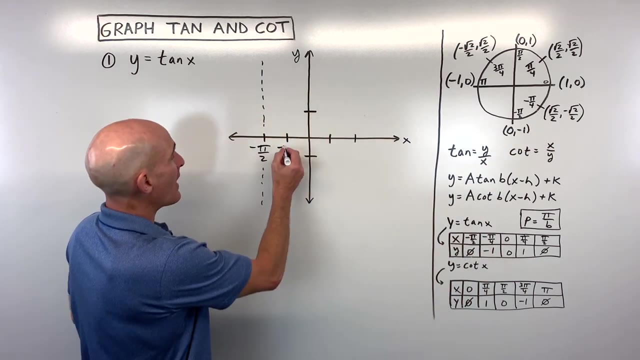 Now at negative pi over 4 or negative 45 degrees. you can see tangent would be negative root 2 over 2, divided by positive root, 2 over 2.. Of course anything divided by itself is 1, and a negative divided by positive would be a negative. So we're getting a negative 1 at negative pi over 4.. 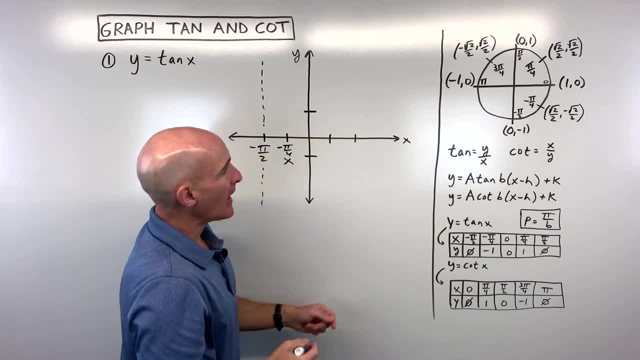 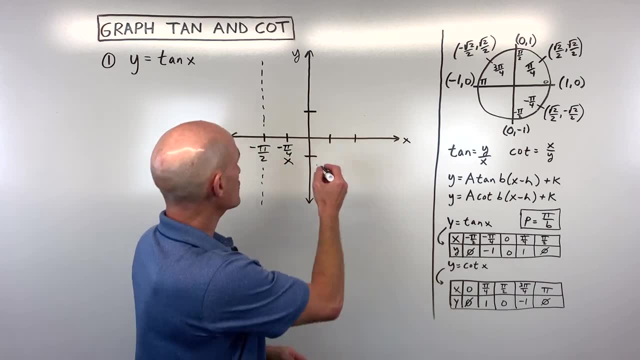 So that's going to put us right about here. And then at 0 tangent is y divided by x, So 0 divided by 1, which is 0.. And so that's going to put us right here at the origin. And then at pi over 4. 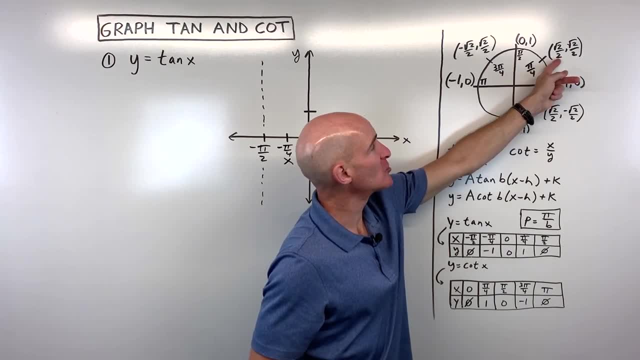 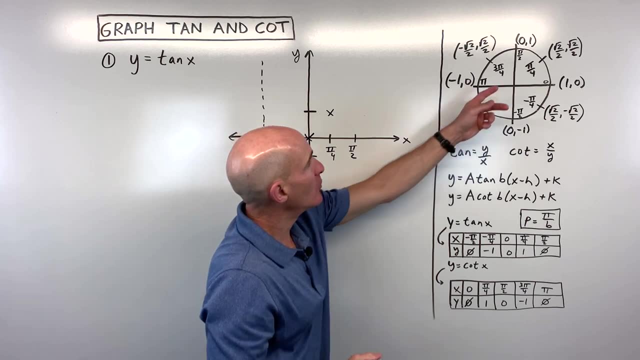 tangent is y divided by x, root 2 over 2. divided by root 2 over 2 is going to equal 1.. So that's going to put us right here. And then, at pi over 2 or 90 degrees, tangent is y over x or 1 divided by 0. We can't divide by 0. So that's going to put us right here. And then at pi over 2 or 90 degrees, tangent is y over x or 1 divided by 0.. We can't divide by 0.. So that's going to put us right here. And then at pi over 2 or 90 degrees, tangent is y over x or 1 divided by 0.. We can't divide by 0. 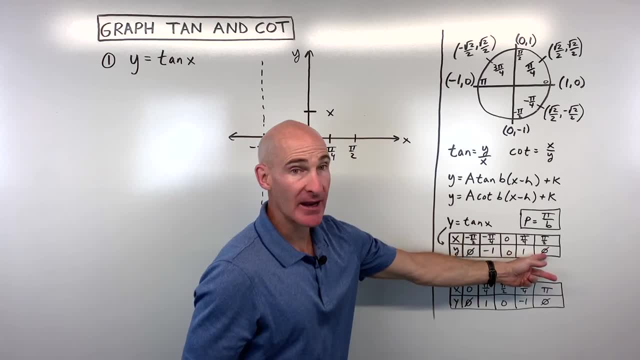 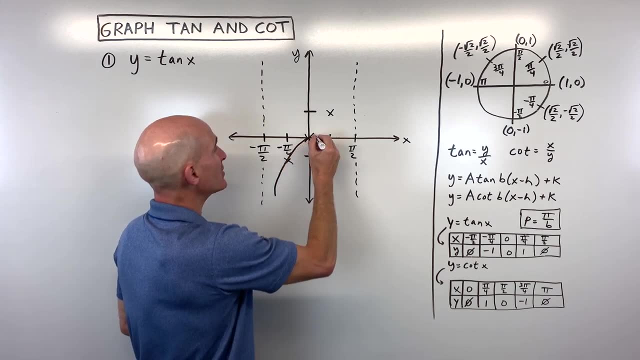 one divided by zero. we can't divide by zero, so that's going to be undefined and we're going to get another vertical asymptote here, and so our basic graph, our parent function, is going to look something like this, where it's approaching the- uh, the two asymptotes, and it's going up to the right. 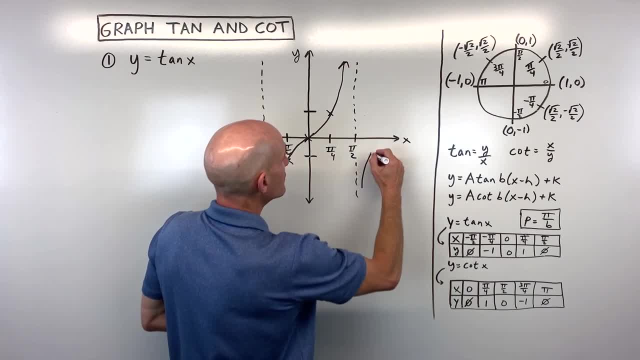 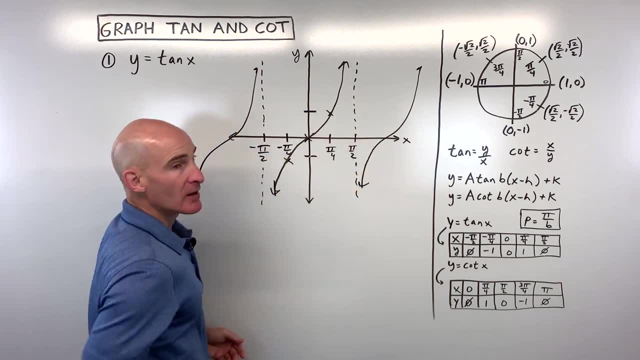 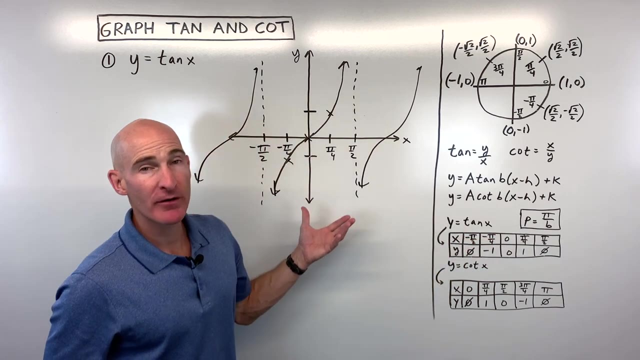 like that and it's going to repeat. so you would have another, you know, branch of the graph like this, another branch of the graph like this, and it's going to repeat with a period of pi, unless it's been stretched or shrunk. and so this is your basic parent function. you want to memorize this. 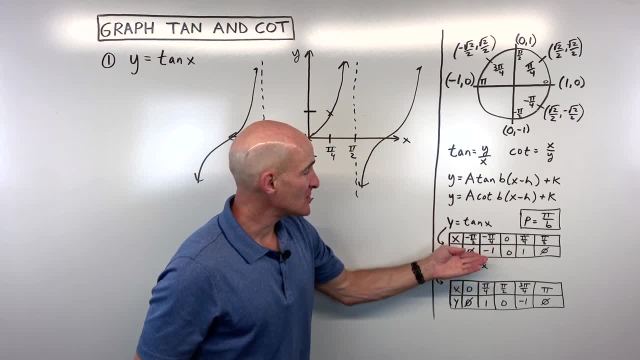 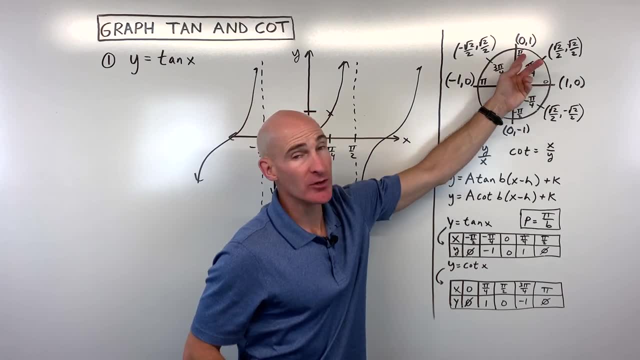 you might also want to memorize these key values, this table here that i've got written. if you forget, you can always go back to your unit circle. just plot the points from negative pi over two to positive pi over two. now let's take a look at some graphs of tangent where it's being stretched. 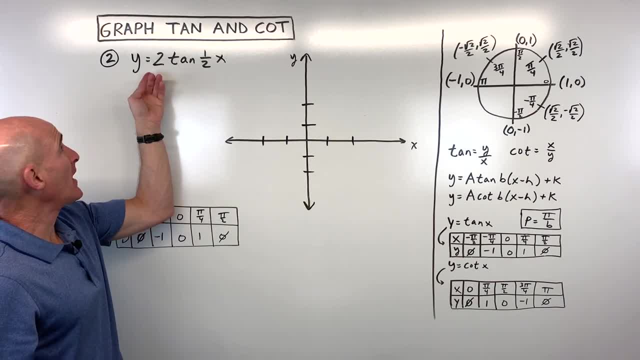 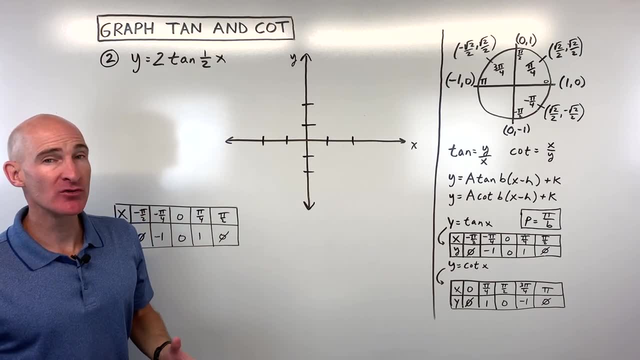 or shrunk, etc. okay, for example, number two. now we're going to graph. y equals two tangent one half x, and i'm going to show you two methods in this video for graphing. some people are going to use method one, some people are going to like to use method number two, which is more like a table type method, but i'll show you. 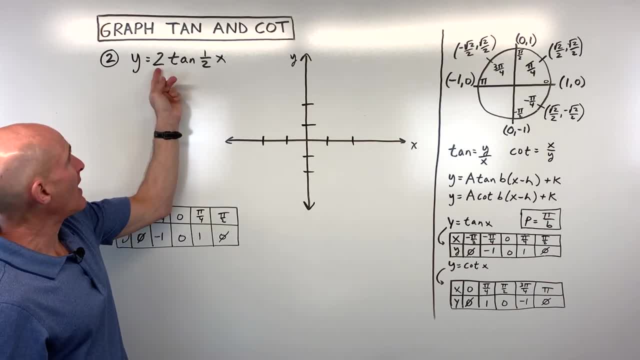 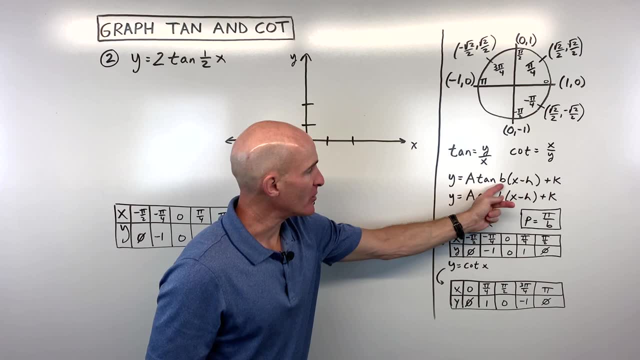 both methods, so you can kind of pick which one you like. now, the way that i learned it when i was learning about graphing tangents and cotangents was we usually started with this b value, right here, the number that comes in front of the x, and what we did is we said: all right, our period is. 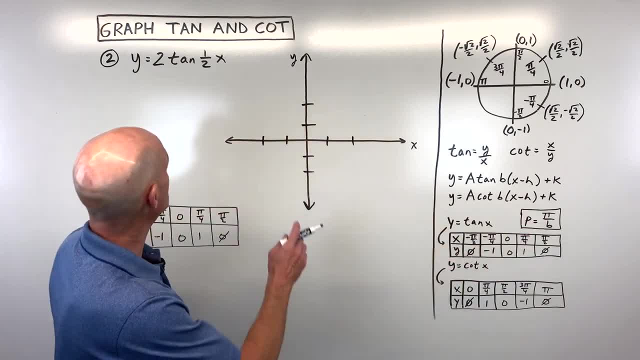 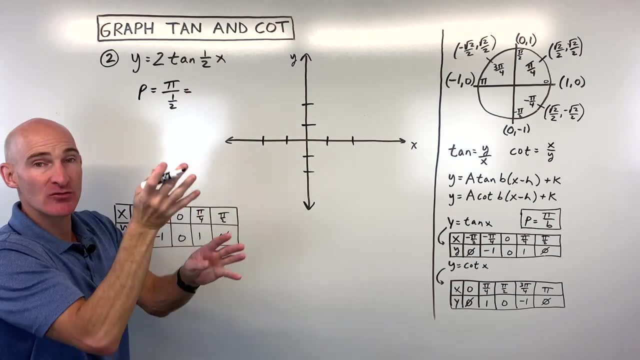 going to be equal to pi over two, and then we're going to take the first one and we're going to divide it by b. so in this case we would say: all right, the period is equal to pi divided by one half. when you divide by a fraction, remember it's like multiplying by the reciprocal, so that's going. 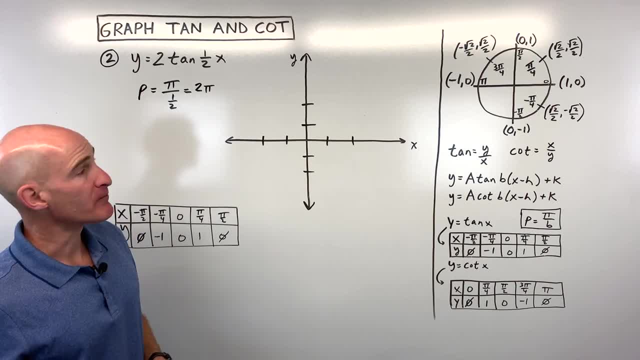 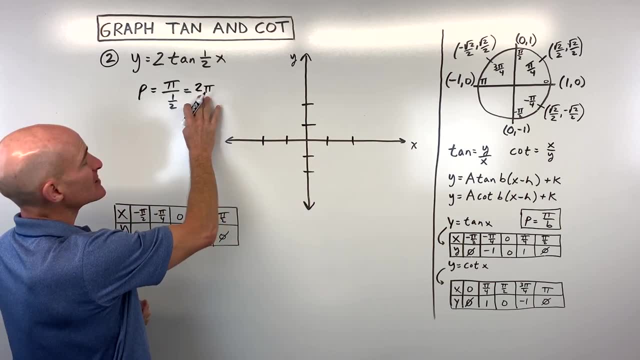 to give you a period of 2 pi. now, if you remember what our parent function looked like, remember how half the graph was on the left side of the y-axis and half was on the right. so what i do is i take this period of 2 pi and i cut it in half. half of 2 pi is going to be pi, so this is going to be. 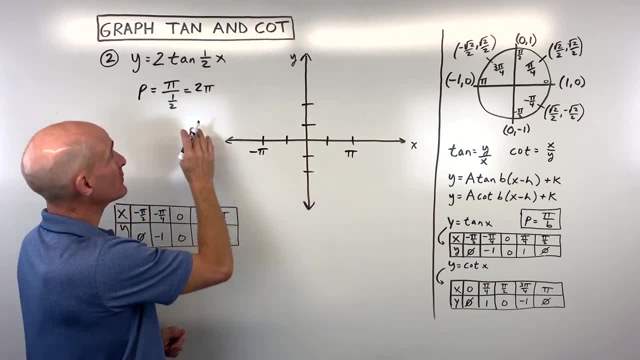 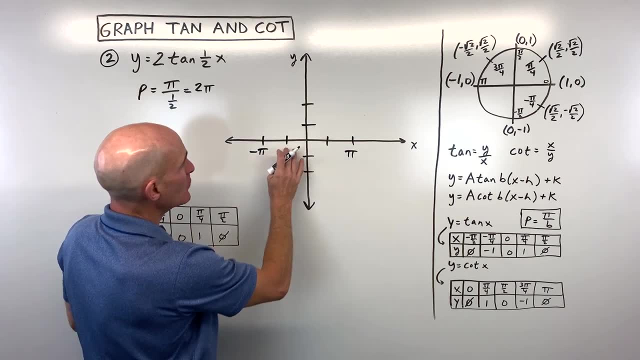 negative pi and pi is going to be negative pi and pi is going to be negative pi and pi is going to be positive pi. that's going to give us a period of 2 pi. see how i split that in half. and then the next thing that we would do is we'd say: well, let's go ahead and find these midway points, so we cut the. 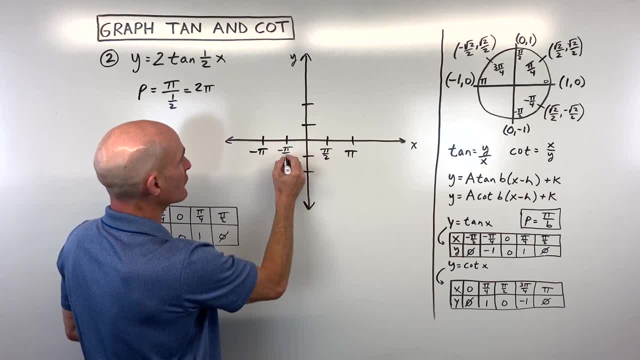 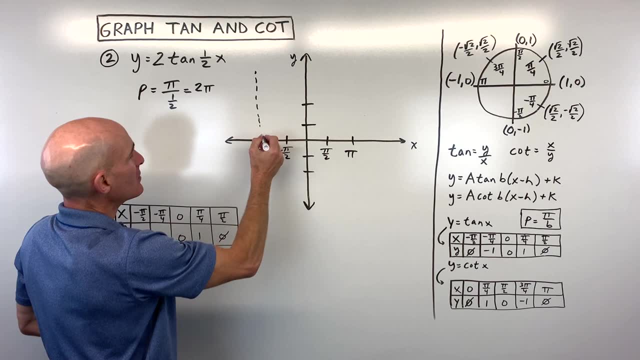 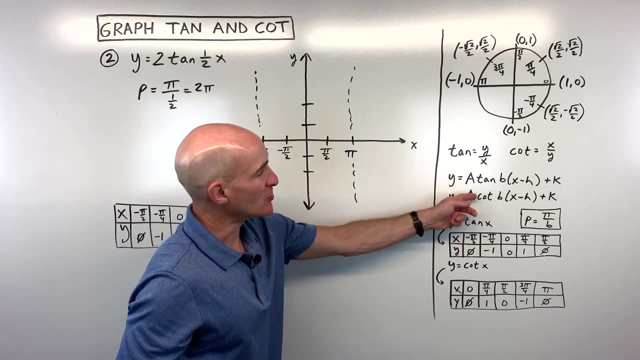 pi in half. so that would be pi over 2 and this would be negative pi over 2.. okay, now what we like to do is go ahead and draw in our asymptotes, which we said are going to be right here at these two values, and then the 2, this a value here in front of the tangent or cotangent, is going to stretch. 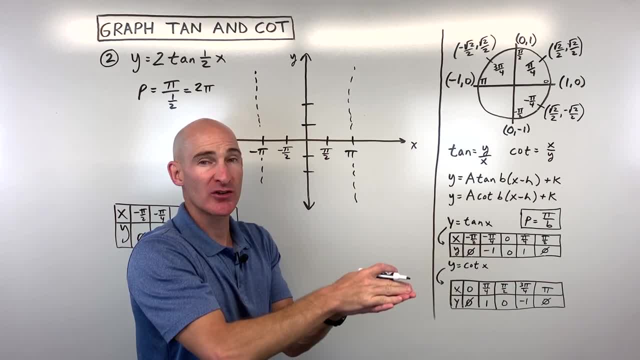 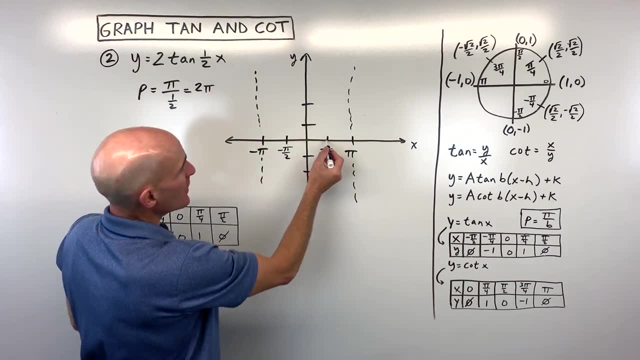 the graph. if it's greater than 1, or if it's between 0 and 1, it's going to shrink the graph vertically. it's going to multiply all the y values by 2.. so this is a vertical stretch by a factor of 2.. so at these, what we used to call these midway points, you're going to be up here at 2 and down. 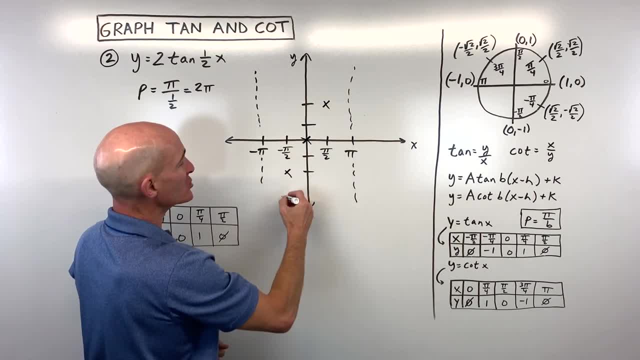 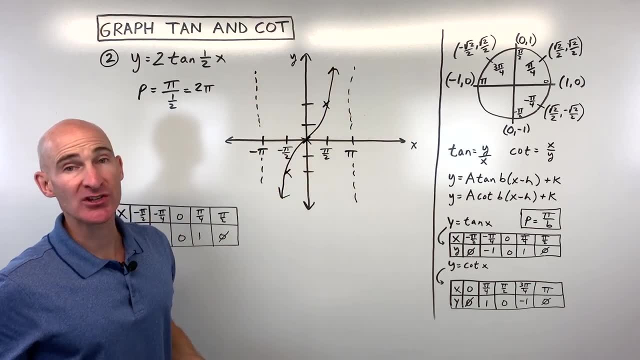 here at negative 2.. that's the stretch and it's going to go right here through the origin and that's going to give us our basic graph and again it's going to repeat, you know, in both directions. so that's one way to do it, that's the way i originally learned it and you might like that. 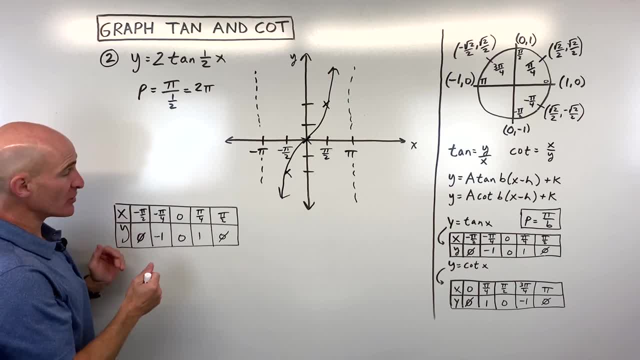 method. if you're interested in learning how to do it, you can go to the link in the description and you can go to the link in the description and you can use that method. but a lot of teachers now are showing this table method using transformations and you might like this a little bit better. 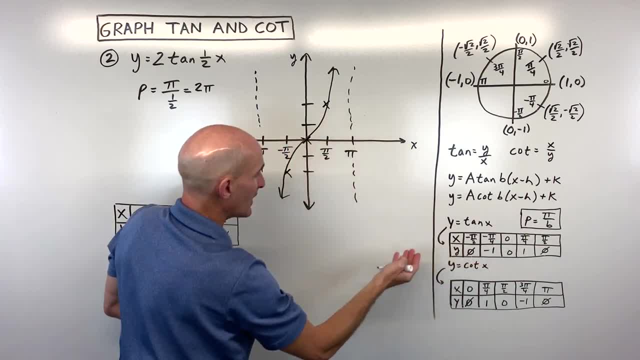 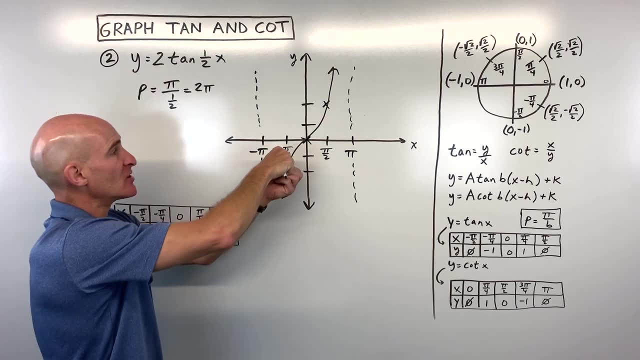 so, again, you might want to memorize these values for tangent, okay, and i just copied that table right here. but now what we're going to do is we're going to use the transformations, we're going to say: all right, this 2 value is going to be a vertical stretch by a factor of 2.. 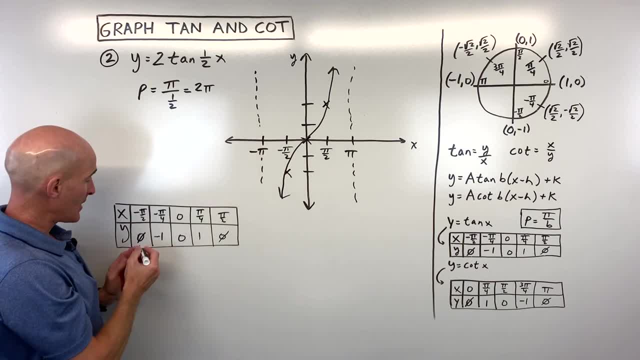 vertical that affects the y values right up and down. so i'm going to multiply all these y values by 2.. well, undefined times 2, we're still going to say is undefined. this is going to be negative 2, 0, positive 2 and still undefined. so i'll just cross out those old y values. all right for the. 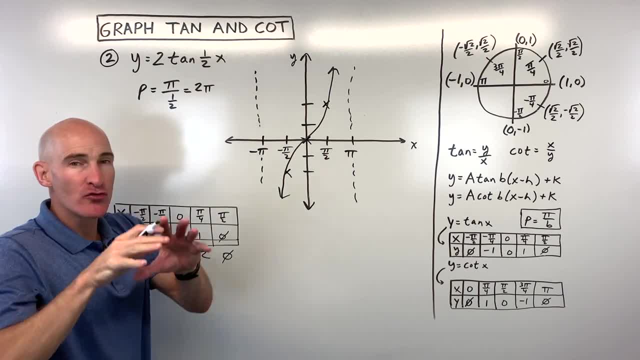 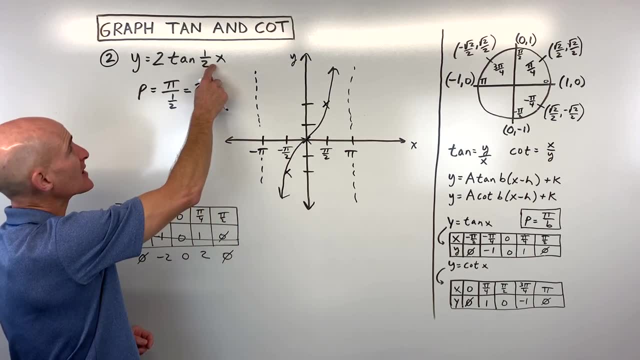 x values. now see this one half, whatever is grouped with the x- okay, with the x- is going to affect the x values, but it's going to have the reciprocal effect. so we're really going to be multiplying the x values not by one half, but by the reciprocal 2 over 1, or you can just say 2.. so when we multiply, 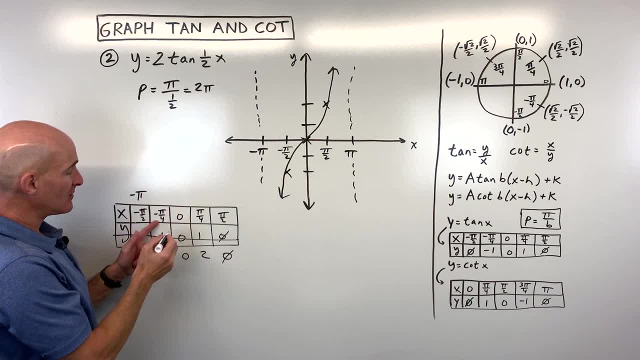 negative pi over 2 by 2, we're going to get negative pi. negative pi over 4 times 2, that's negative. pi over 2: 0 times 2 is still 0. pi over 4 times 2 is pi over 2 and pi over 2 times 2 is pi. let's cross. 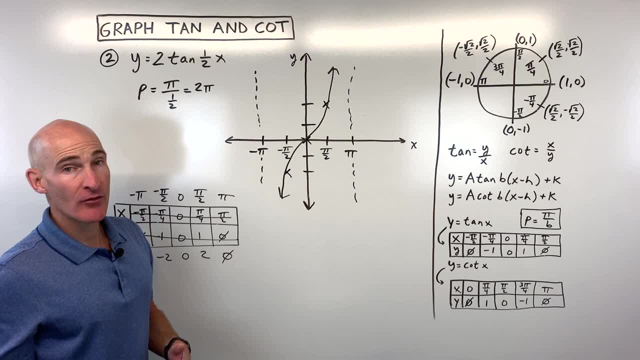 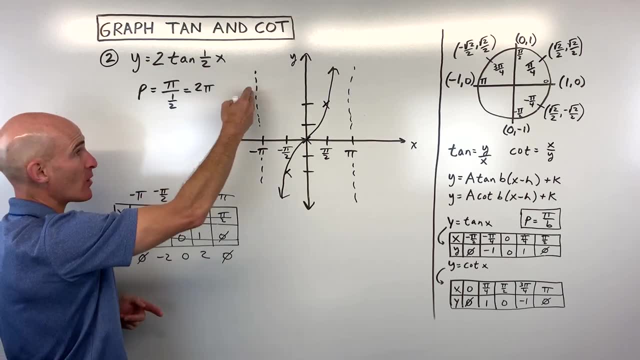 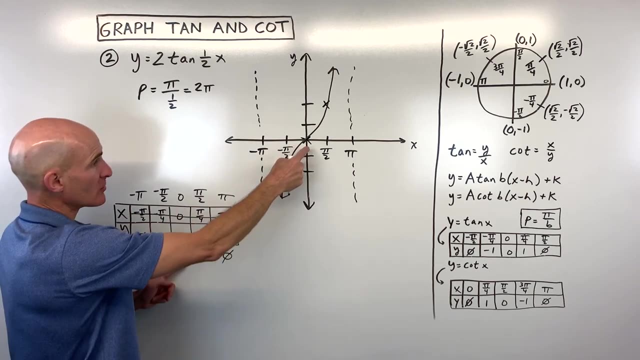 out those old x values. now we've taken care of our transformations, we can plot these values so we can say: at negative pi, see it's undefined. and that's why we have that vertical asymptote here. at negative pi over 2, you can see we're at negative 2, at 0, we're at 0. that's the origin at pi over 2. 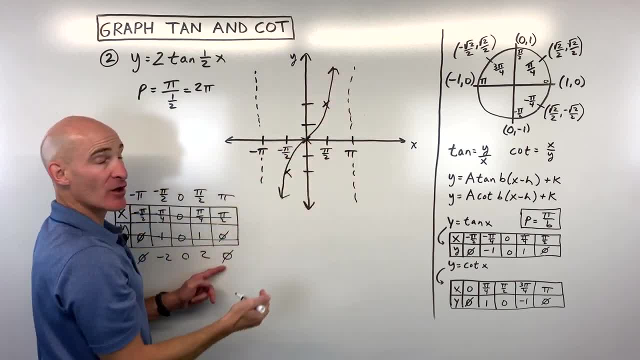 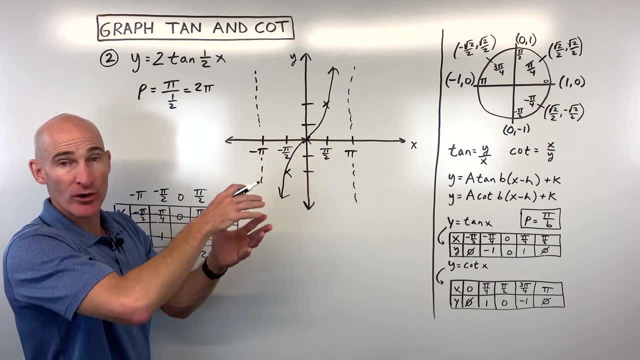 at 2 and at pi it's undefined. we get another vertical asymptote. so two different methods you can use. you know kind of like knowing the parent function and kind of working with that parent function, or you can work with the table. let's take a look at another example, okay, for example: 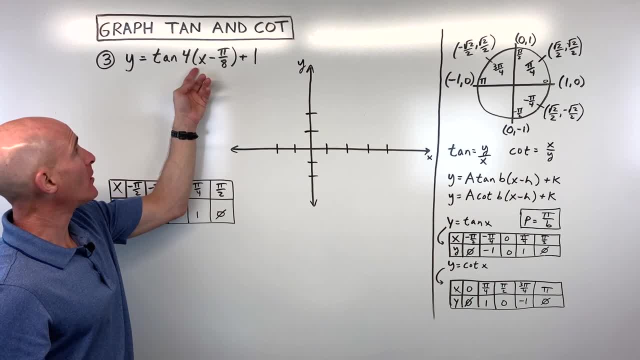 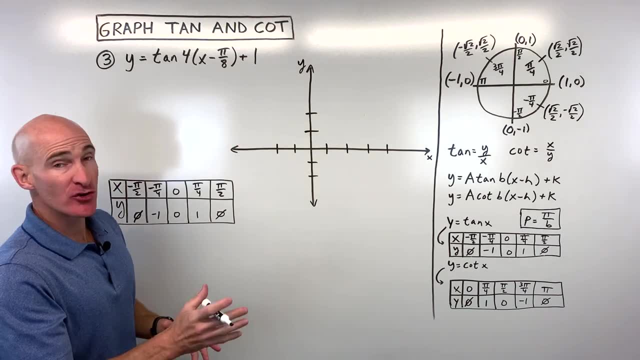 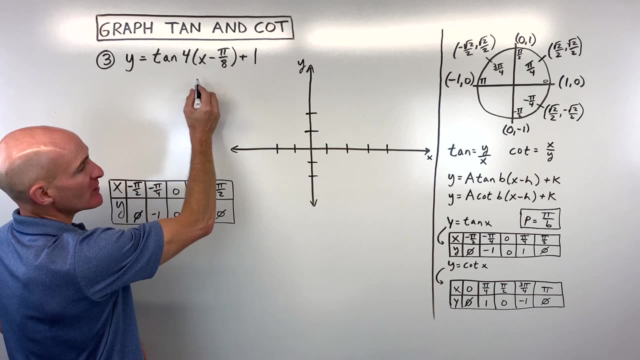 number three. now we have y equals tangent 4 times the quantity x minus pi over 8 plus 1.. how would we graph that one? well, i'm going to show you method number one, kind of the way that i learned back in the day, and i would start with this b value. okay, so the b value is a number that comes just. 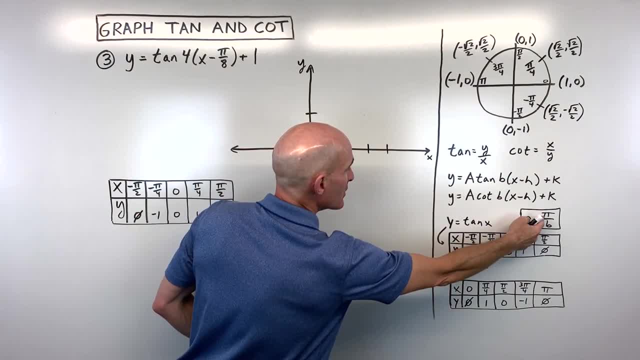 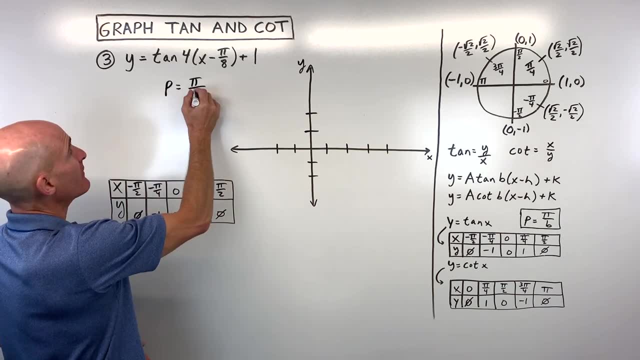 to the left or in front of the x and we use this formula: period equals pi divided by b. so i would say the period is equal to pi. that's the normal period for tangent divided by 4.. now i'm going to use that technique of cutting that pi over 4 and 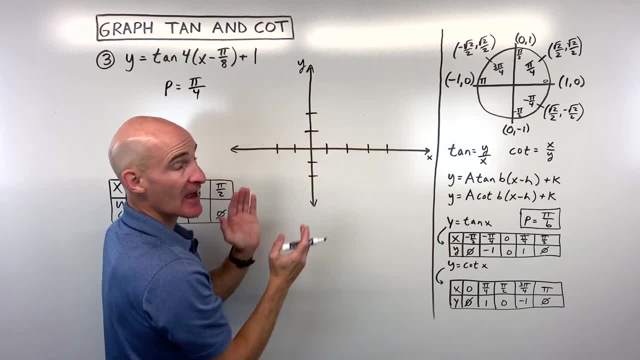 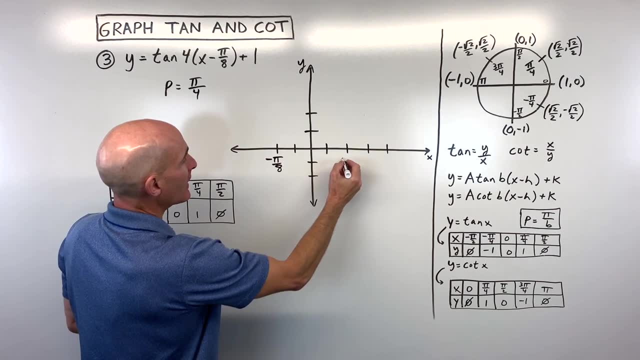 half, because remember how half the tangent graph was to the left of the y-axis and half was to the right. so half of pi over 4 is going to be pi over 8. so i'm going to say negative pi over 8 and positive pi over 8.. And then what I'm going to do is I'm going to find 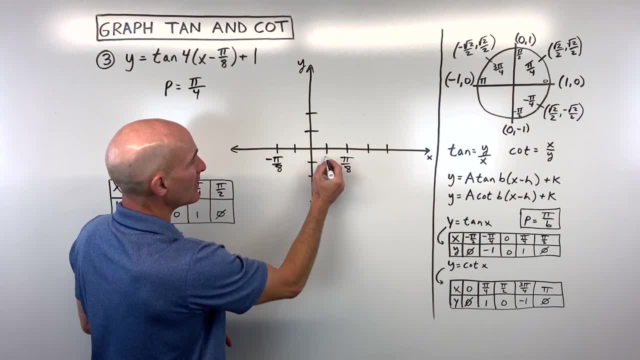 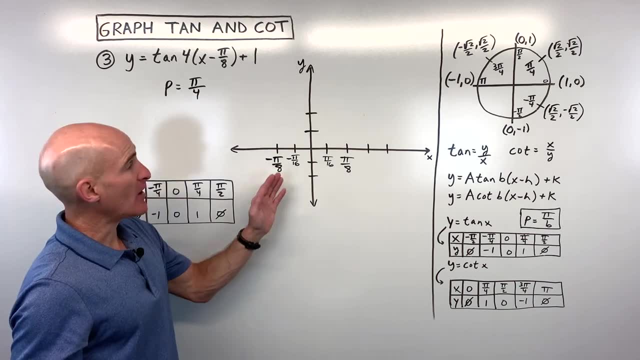 these midway points, these halfway points, by cutting pi over 8 in half. That's going to give us pi over 16. And over here we'll have negative pi over 16.. So that's how I set it up. So now I 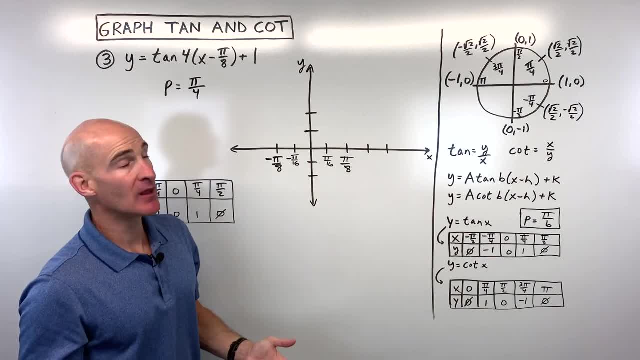 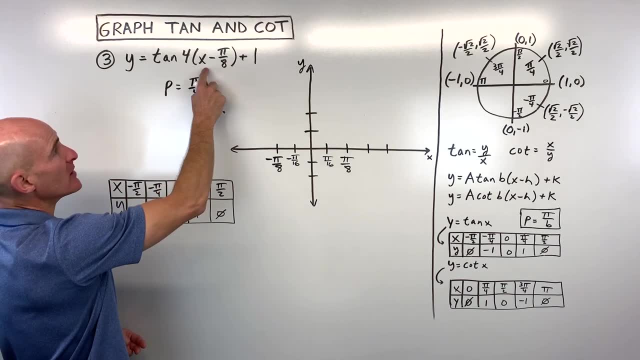 know what my scale is. I'm counting by pi over 16s each time. Okay, then what I would do is I would look at this shift here. I say okay, minus pi over 8 and plus 1.. So when you add or subtract, 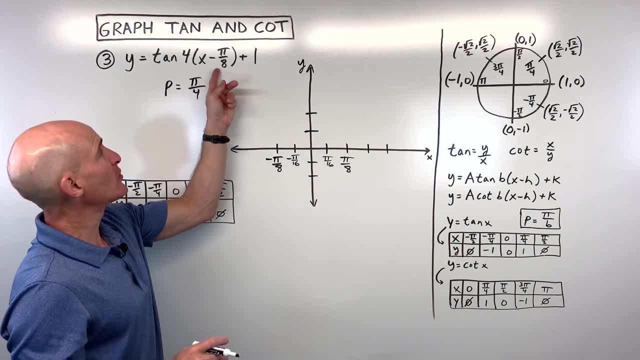 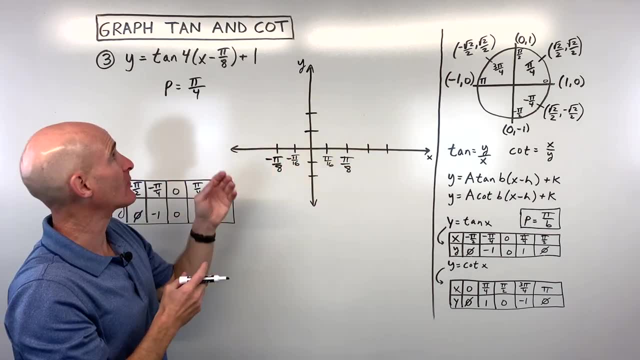 that's like a translation or a shift. Whatever is grouped with the x, remember, it has like the opposite effect. If it's minus, you're actually going to go positive to the right, If it's plus, you're actually going to go negative to the left. So in this case, the minus pi over 8 means we're. 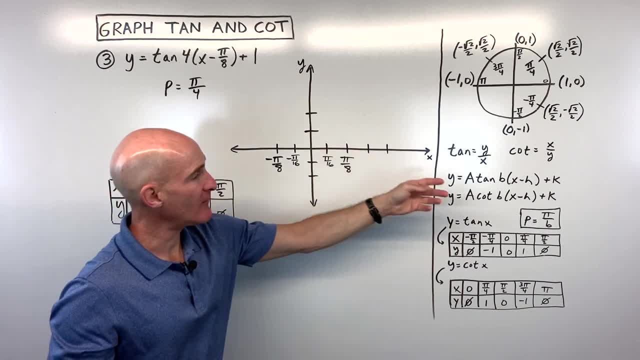 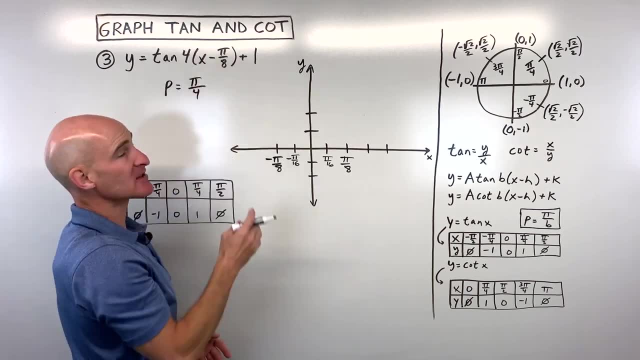 going to shift right pi over 8. And the plus 1, this k value here, is going to shift the graph up or down. Positive you go up, negative you go down, It has the same effect. So I usually think whatever's grouped with the x, opposite effect. Whatever's not grouped with the x, same effect. 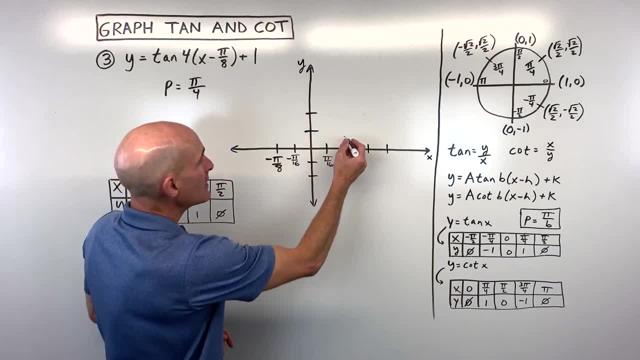 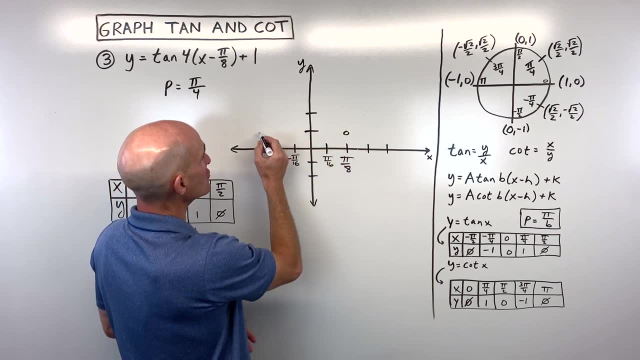 So minus pi over 8 goes right: pi over 8. Up 1.. So what I'm going to do is I'm going to think of this point right here as like my new origin, Instead of here. this is going to be like our new origin, So what I'm going to do is I'm 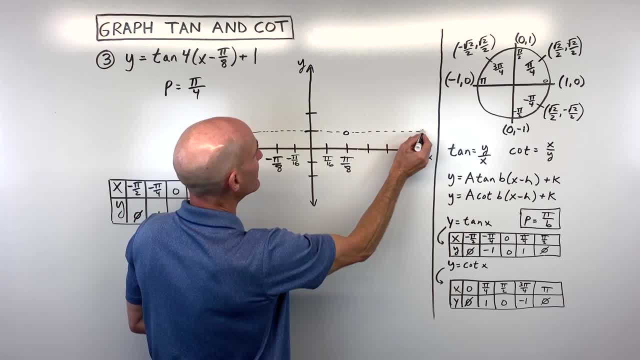 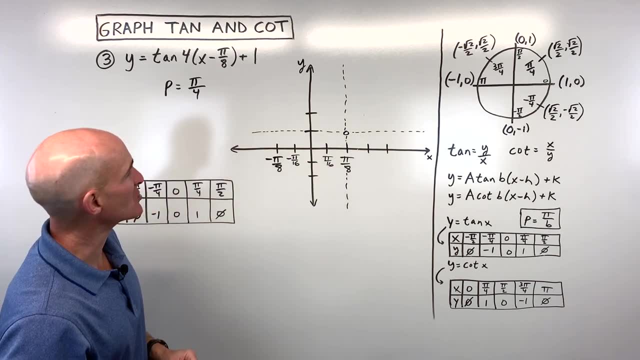 just going to draw in a little dotted line, kind of like this, just to kind of think of this as my new x and y axis. Okay, they're not asymptotes, just kind of thinking of that as our starting point. Then what I would say is I'd say, okay, this a value is like our stretch or our shrink. 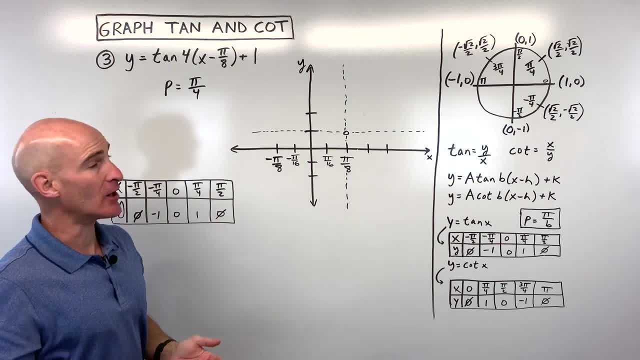 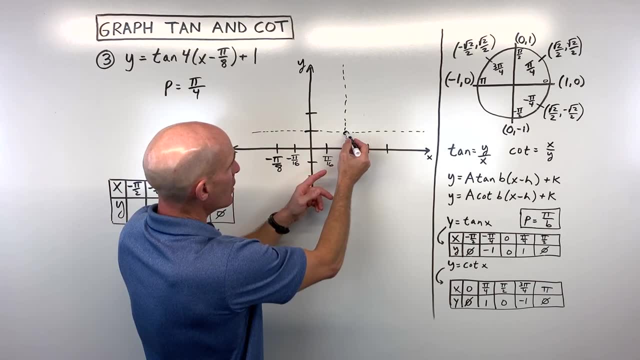 In this case, the a value is just 1.. So it's really not stretching or shrinking at all. It's just going to be the normal tangent graph where you go at the midway points up 1.. So what I would do is I would say: okay with tangent, I know it goes right through the origin. 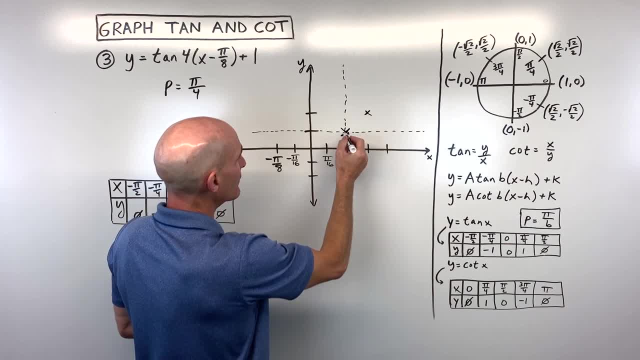 At the midway point I know that I'm going to be going up 1. And if I go the other direction, I know I'm going to be going down 1.. And then I have my asymptotes right here. So this is going. 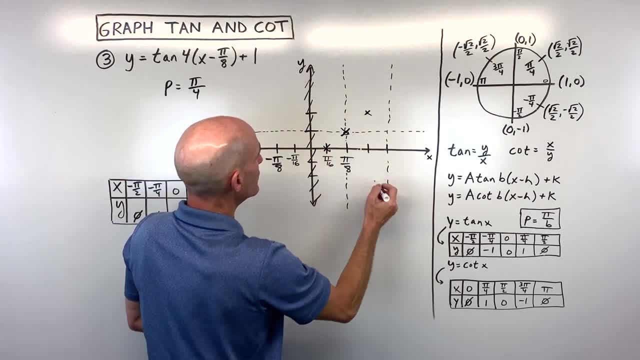 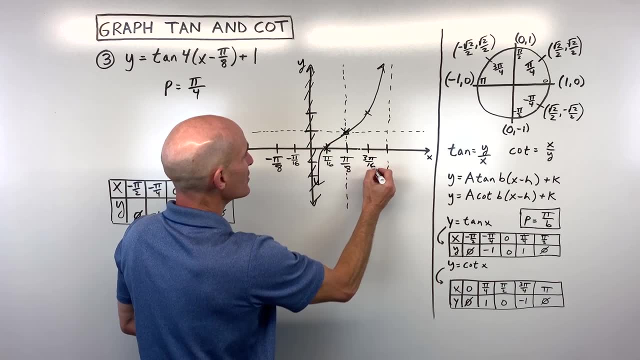 to be right here and right here, And then I've got my graph like this. Now you might say, Mario, that was kind of confusing, Like what was all of that. Or some of you might say, oh, that was that makes complete sense. That's how my teacher 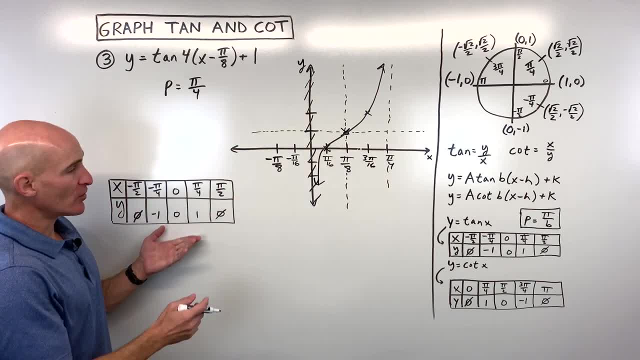 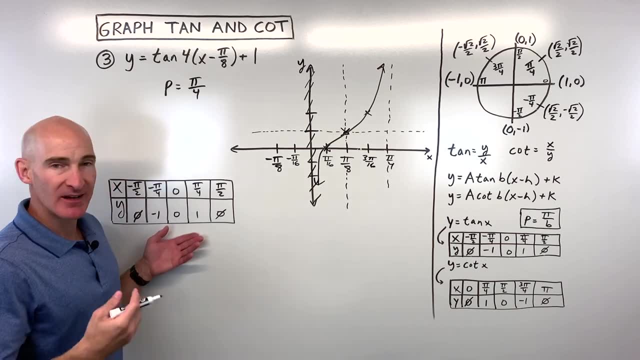 explained it right. But let's look at method number two, using the table. So again, I'm just using these values. You might want to memorize these values. Again, they come from the unit circle, if you forget. But after you write them down a few times, you'll commit them to memory. 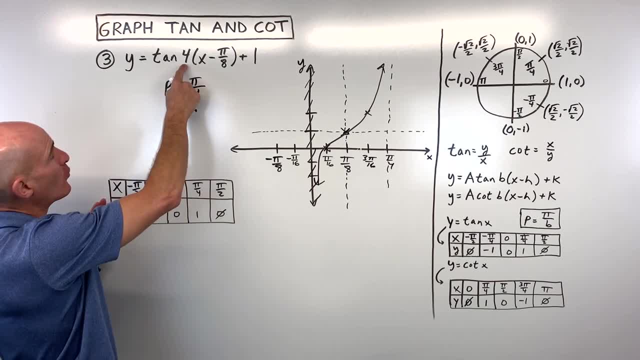 So we're starting with this table And what I would do is I would start with this 4.. I'd say, hmm, what is this 4? due to the graph? Well, it's grouped with the x, It's going to have the 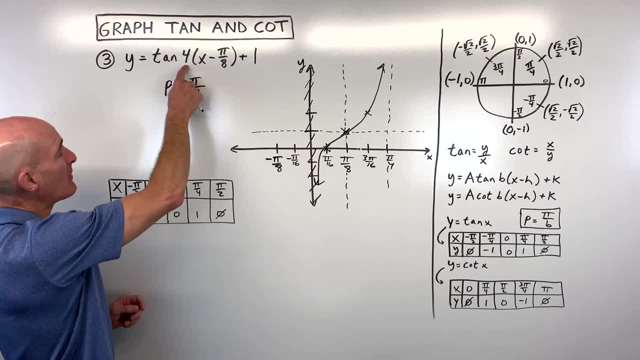 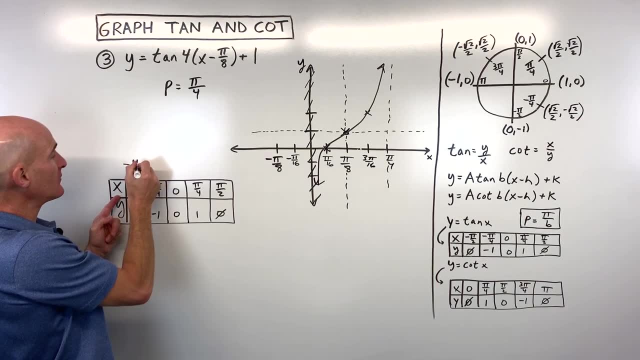 reciprocal effect. So it's going to multiply all the x values not by 4, but by 1 fourth. So on this table I'm going to multiply all my x values by 1 fourth. That's going to give you negative pi. 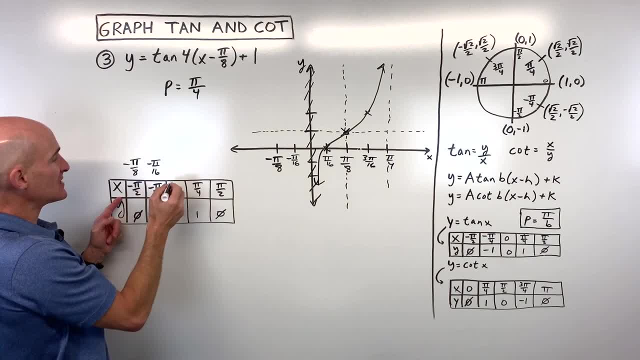 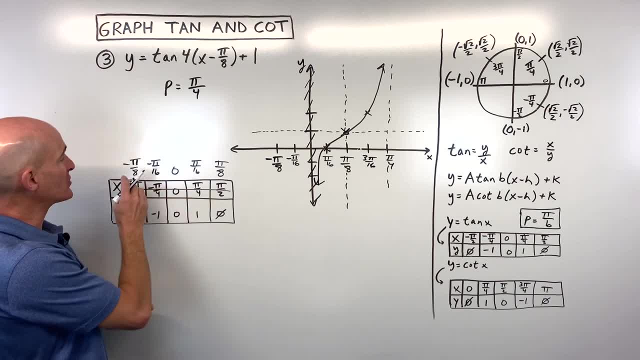 So I'm going to be adding pi over 8 to all of these x values. So if I do that, that's going to put us at 0.. That's going to put us at pi over 16.. That's going to put us at pi over 8.. 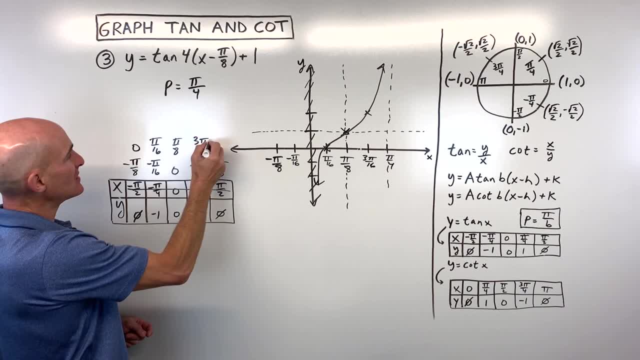 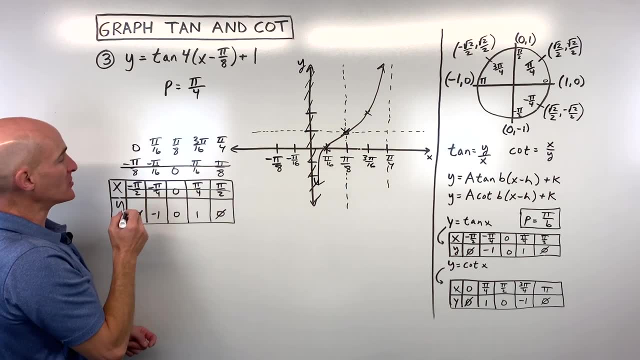 That's going to put us at 3, pi over 16 and that's going to put us at pi over 4.. I'm going to cross out those old x values, Okay. and then, lastly, this plus 1 is going to shift the graph up: 1.. 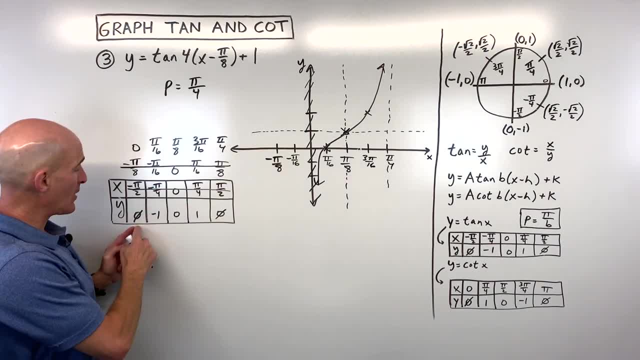 And so that affects the y values when you shift up or down. So I'm going to add 1 to all my y values here. Of course, undefined plus 1 is still going to be undefined. Native 1 plus a 1 is 0.. 0 plus 1 is 1.. 1 plus 1 is 2. 0. 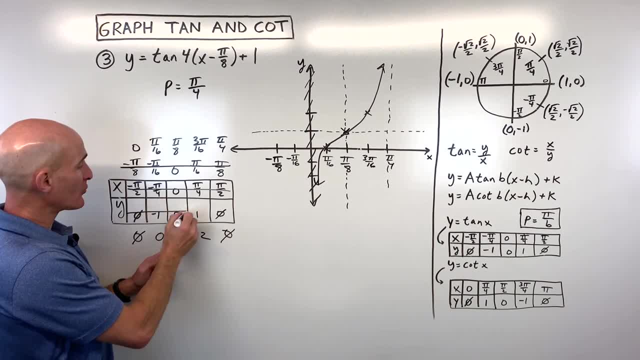 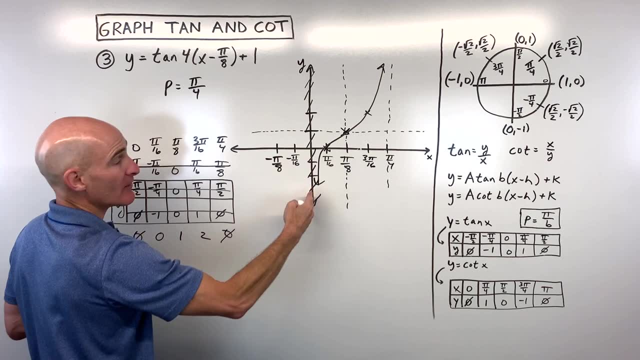 are undefined, plus 1 is still going to be undefined, So we'll cross out those old y values. So now we've got everything we need. We've got at 0. it's undefined, So at 0 we have that vertical asymptote. 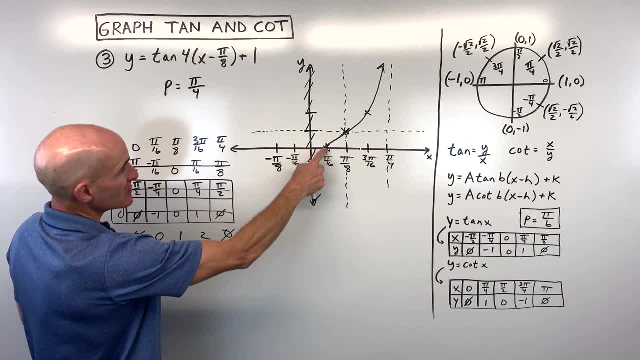 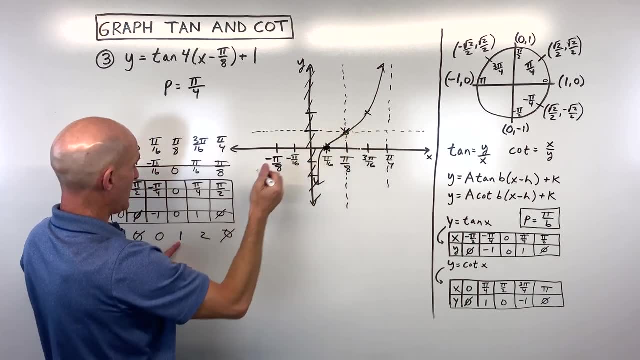 At pi over 16, you can see, we're at 0.. So there's our point right here, See. And at pi over 8, we're at 1.. Okay, which is right here. And then at 3 pi over 16, we're at 2.. That's perfect. 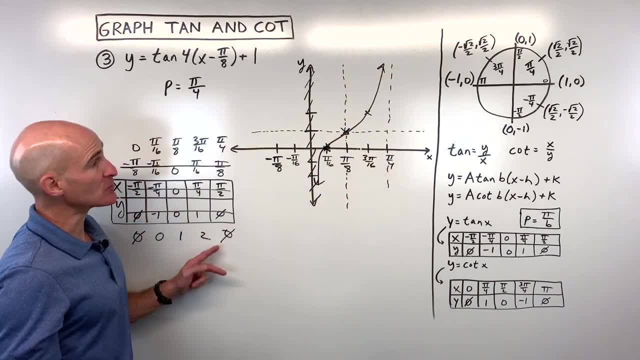 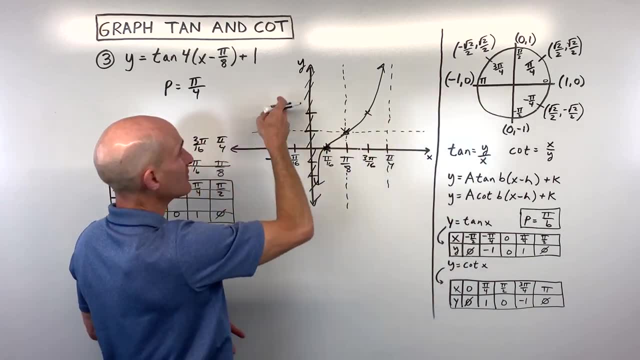 And then at pi over 4 it's undefined. We get another vertical asymptote. Once you get one period or one cycle of the graph, it's pretty easy to repeat and you can just kind of keep going. You know like that Now. 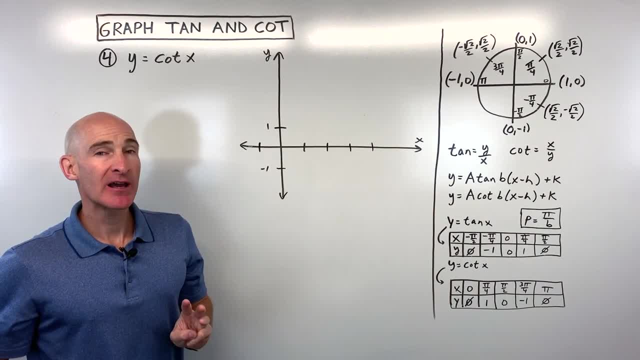 let's take a look at another example. We did three examples talking about tangent. We're going to do three examples talking about the cotangent And then, at the end of this video, I'm going to have two more examples. I'm going to encourage you to try to practice on your own and we'll go through them together: One tangent and one cotangent. 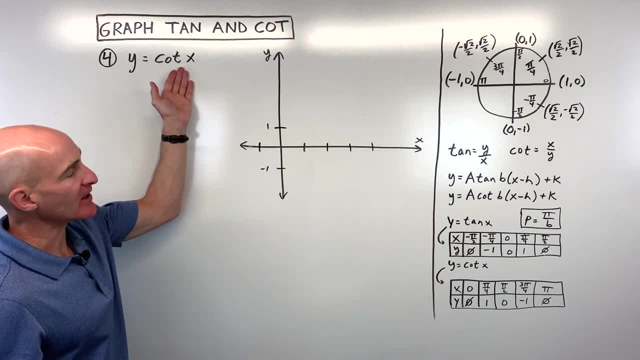 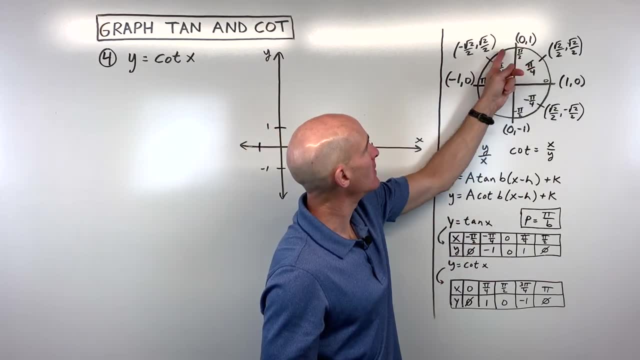 So switching gears for a moment let's talk about cotangent of x. So cotangent of x. when we make a table here of our parent function, we're going to use the values from 0 to pi. Remember, with tangent we went from negative pi over 2 to positive pi over 2.. But for cotangent, 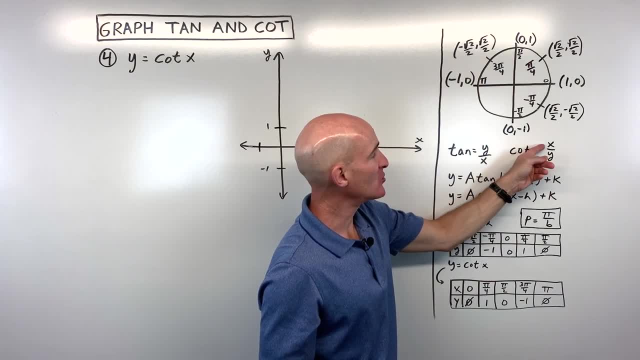 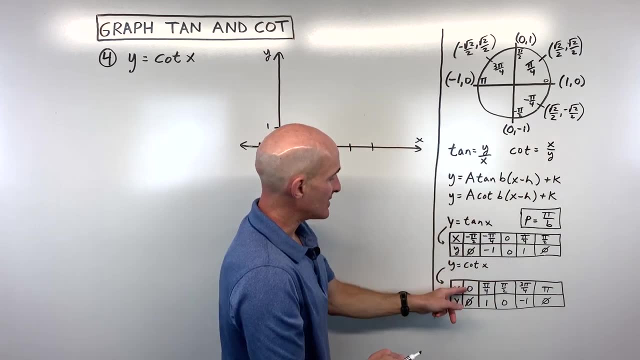 we're going to go from 0 to pi And remember cotangent on the unit circle is equal to the x coordinate Divided by the y coordinate. It's the reciprocal of tangent. So, starting over here at 0, cotangent is going to be 1 divided by 0, which is 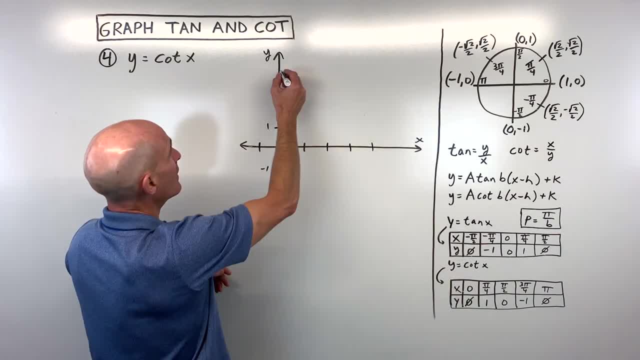 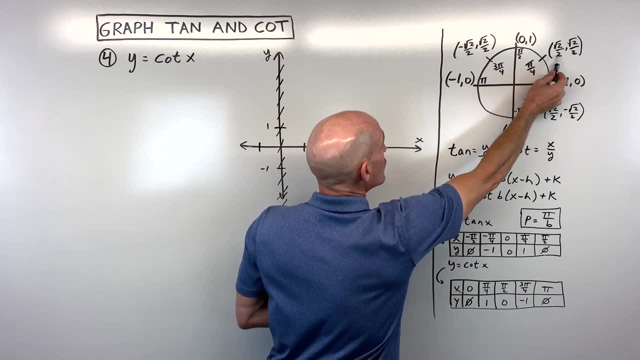 undefined. So over here at 0,. undefined means we're going to have a vertical asymptote, So I'll just draw that as a dashed or dotted line. At pi over 4, cotangent is x divided by y Root 2 over 2. divided by root 2 over 2 is 1.. So you can see here in our table: pi over 4. 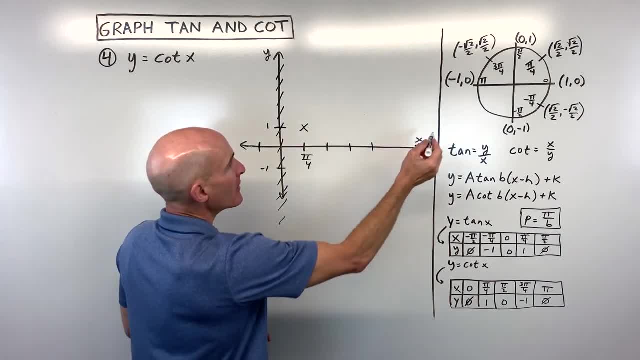 is equal to pi over 4.. So we have: 2 over 1 is equal to 1. And we'll put a point right there. Then, at pi over 2, cotangent is x over y, So 0 over 1 is equal to 0.. 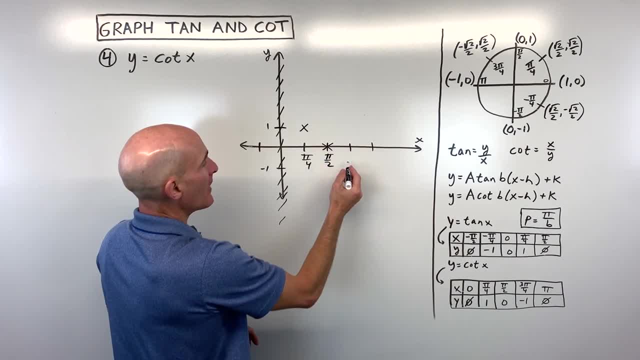 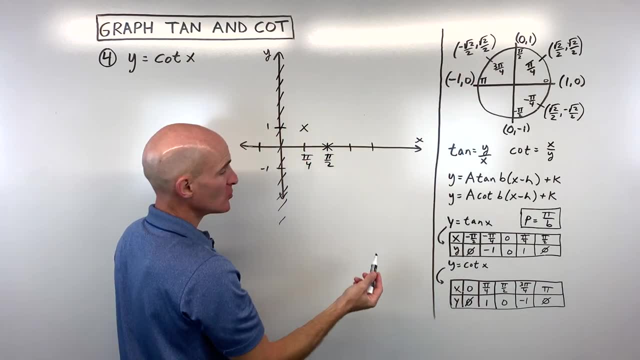 Okay, so let's write that down. pi over 2 is 0.. And then at 3pi over 4, cotangent is x over y. So negative root 2 over 2 divided by positive root 2 over 2 is negative 1.. 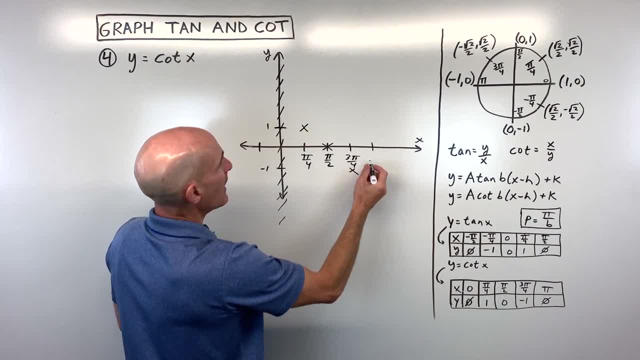 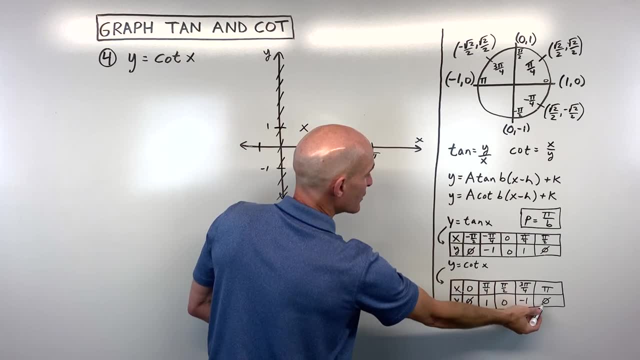 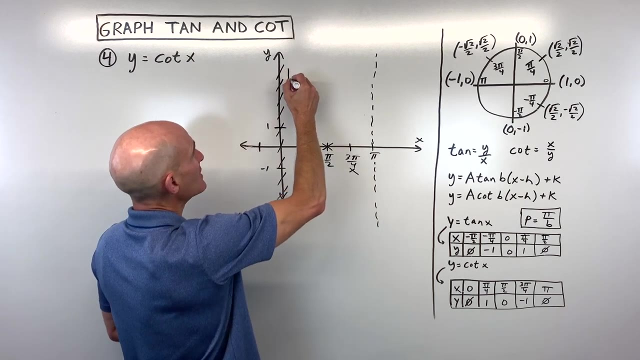 So that's going to put us right down here. And then at pi, which is right here, cotangent is x over y. 1 divided by 0 is undefined, because we can't divide by 0. So that's going to give us another vertical asymptote right here. So our cotangent graph is going to: 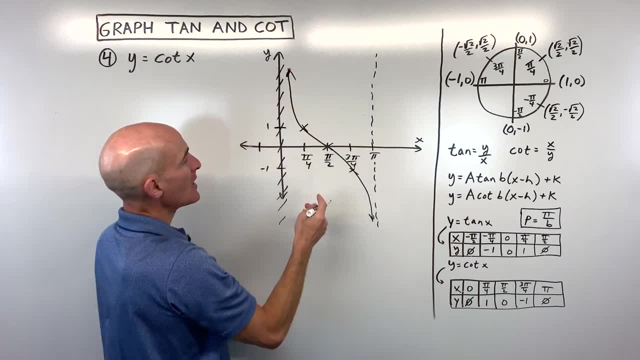 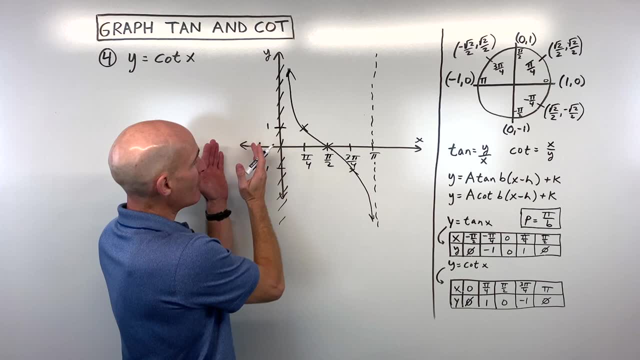 look like this where it's approaching both of the vertical asymptotes, but notice, cotangent is going down to the right. Remember tangent went up to the right and remember tangent, half the graph was on the left side of the y-axis, half was on the right, whereas here, with cotangent, the graph is all to the right. 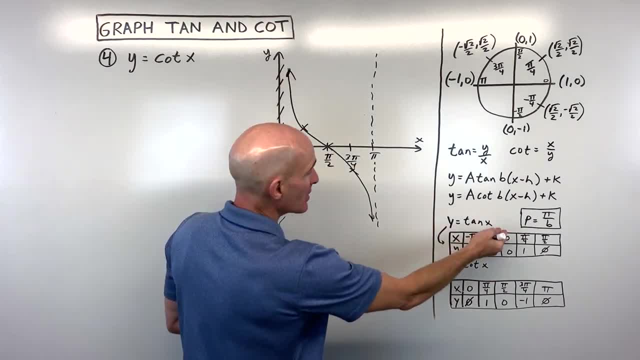 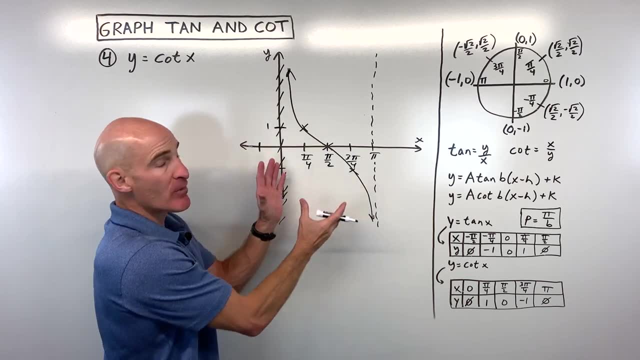 of the y-axis and again it has the same period. just like with tangent, the period is pi. cotangent, the period is pi, you know, unless it's been stretched or shrunk. That's your parent graph, so you want to memorize this and have a good 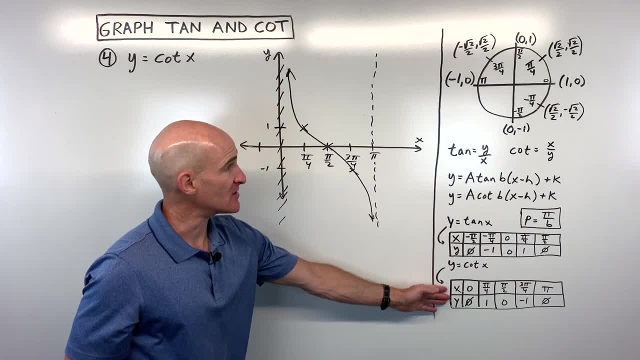 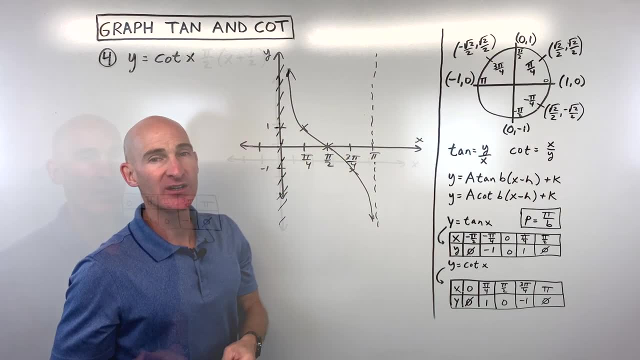 feel for the basic shape and also I would memorize these values in this table. Again, you can recreate it from the unit circle going from 0 to pi. Let's take a look at another example of cotangent. Okay, now in example number 5. 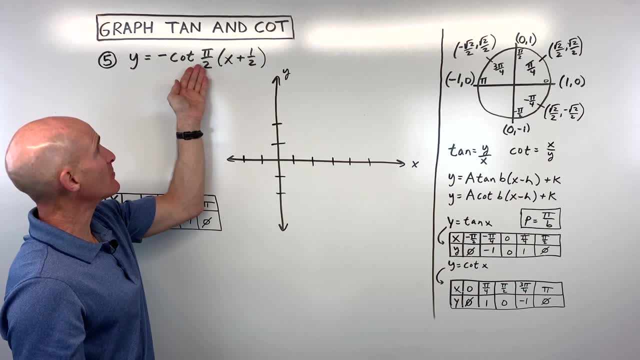 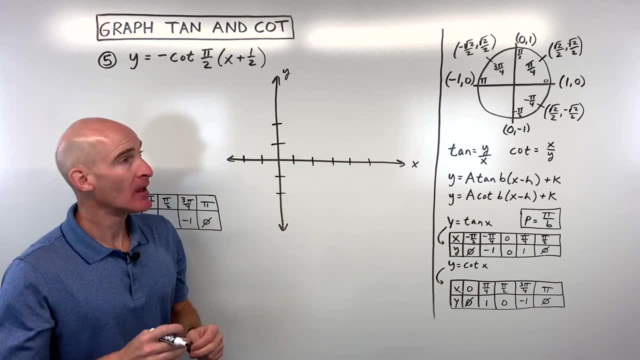 we were trying to graph. y equals negative cotangent pi. pi over 2 times the quantity x plus 1 half. So how would we graph that one? Two methods. Let's do the first method, my old school method that my teachers in high 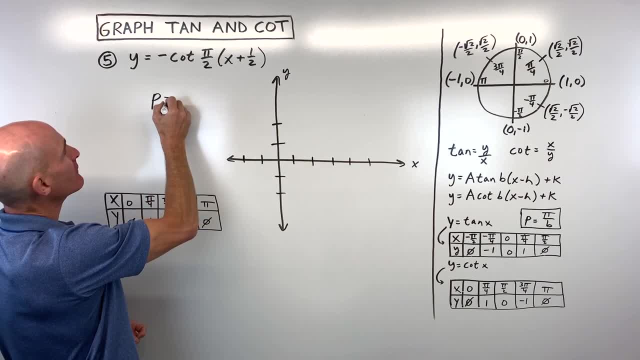 school showed me, which is: hmm, how do I find the period? Well, the period we know for tangent and cotangent is pi, but in this case it's going to be pi divided by our b value, this number that comes in front of the x, and so that's pi divided by pi. 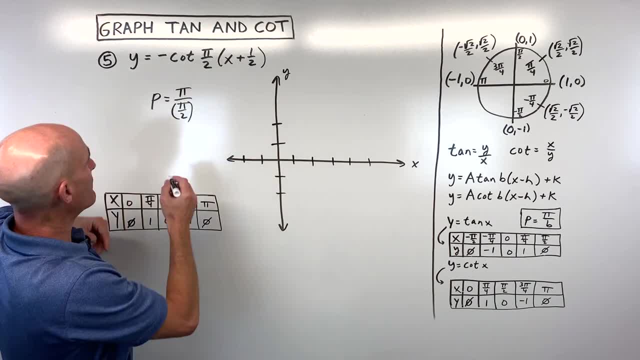 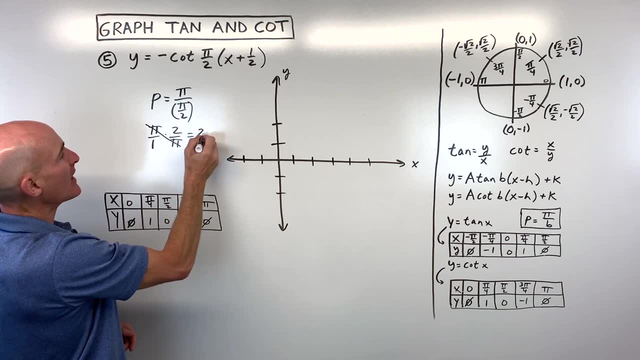 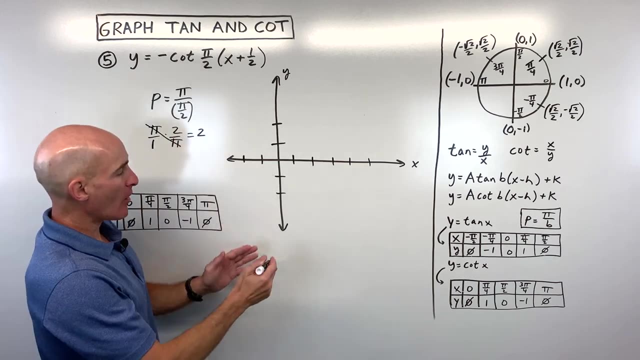 over 2.. Now, when you divide by a fraction, it's like multiplying by the reciprocal. Now this is going to be pi times two over pi, The pi's cancel, And so we're getting a period of two. Okay, so that's interesting. now remember with cotangent, remember how our graph 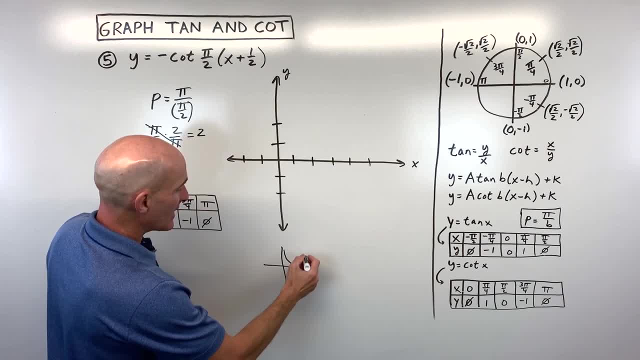 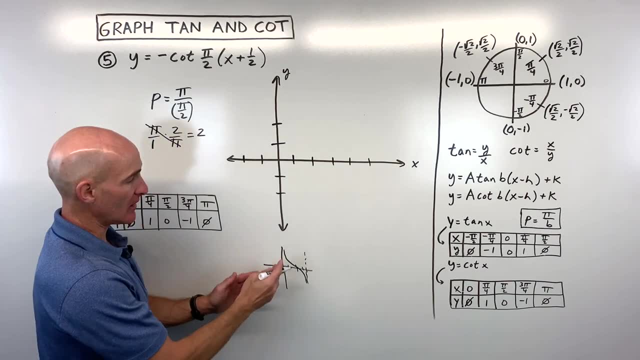 let's just draw a little sketch of our graph. look kind of like this, and I divided it up into four pieces. It was like one, two, three, four, Okay, like four segments, And so what I'm gonna do is I'm going to take this to and I'm going to do: the same thing, I'm gonna divide up into four pieces. This was like one, two, three, four. Okay, so I'm going to do four pieces And this is going to be pi, and this is going to be pi times two divided by pi. 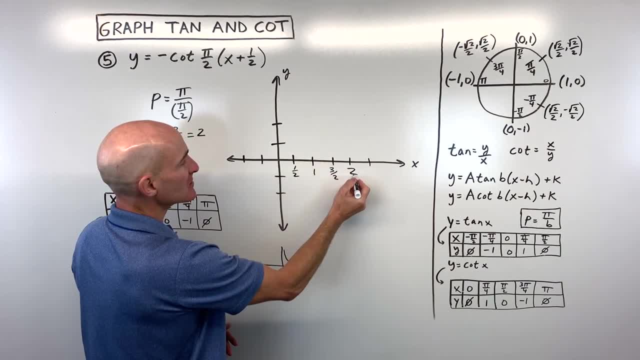 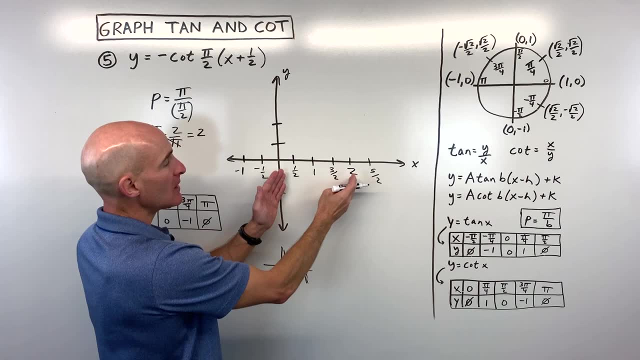 So that's going to be 1 half 1,, 3 halves 2, 5 halves negative, 1 half negative 1.. Once I divide it up by 4, like that, I get my scale. I'm counting by 1 half. 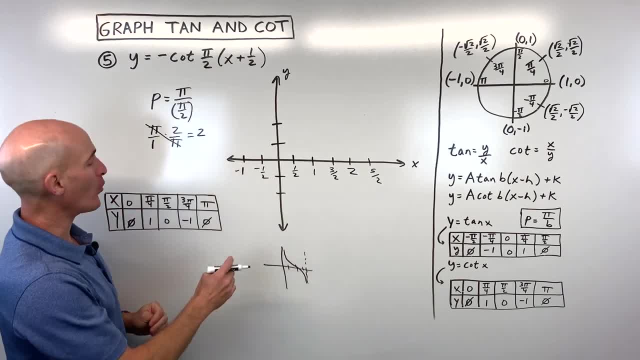 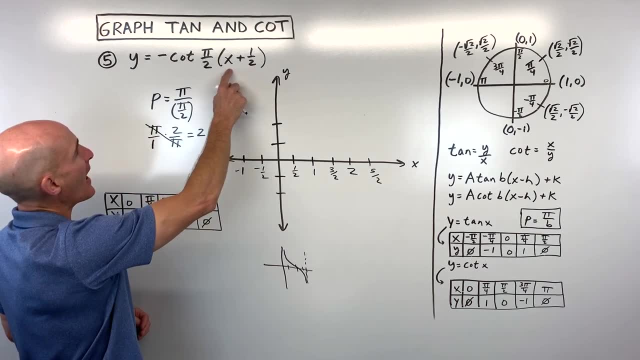 Then you can kind of repeat that process. So just dividing it by 4, dividing it into 4 pieces. Now, once we have the scale, now let's take a look at our shift. So this plus 1 half is going to be shifting the graph not to the right 1 half, but the opposite. 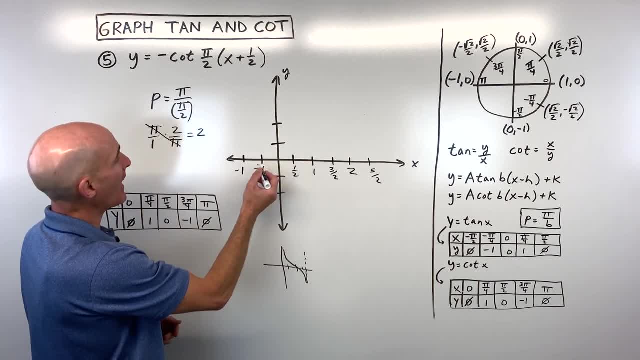 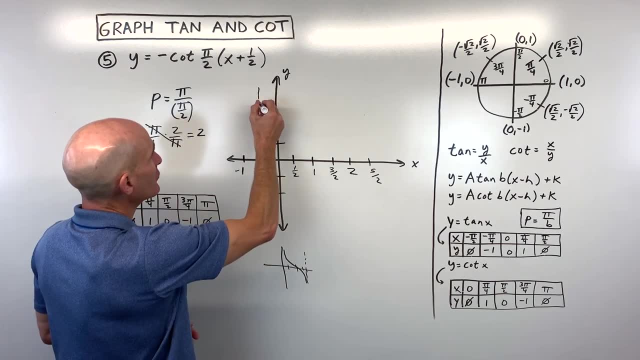 Whatever is grouped with the x has the opposite effect. So we're going to shift it to the left 1 half. That means we're going to think of this right here as our new origin. So you can kind of let's draw in like a little dashed or dotted line here. 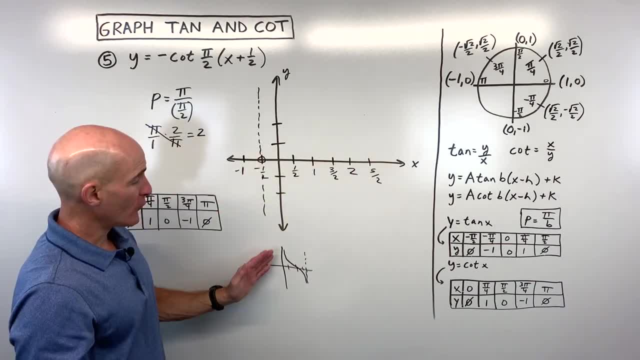 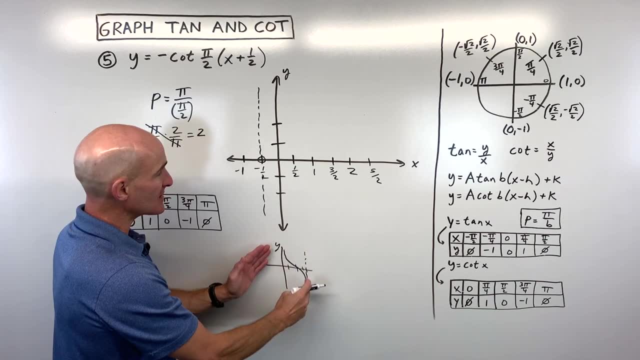 And same thing here. So this is going to be like our starting point Now. if you have in your mind the basic shape of cotangent graph, you can see it's going down to the right. It's to the right of the y-axis. 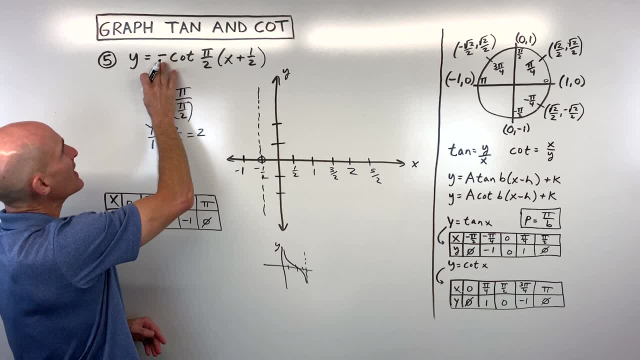 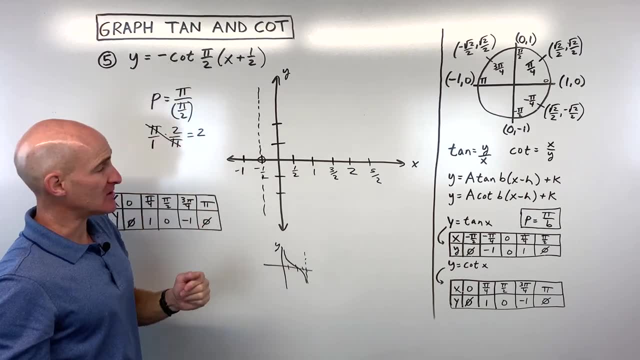 Okay, but this is kind of like our new y-axis. And then what does this negative here do? Well, the negative is going to. it's going to reflect the graph over the x-axis. It's going to make all the y-values the opposite, right? 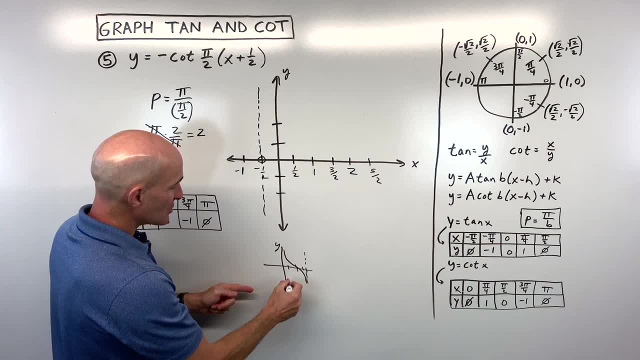 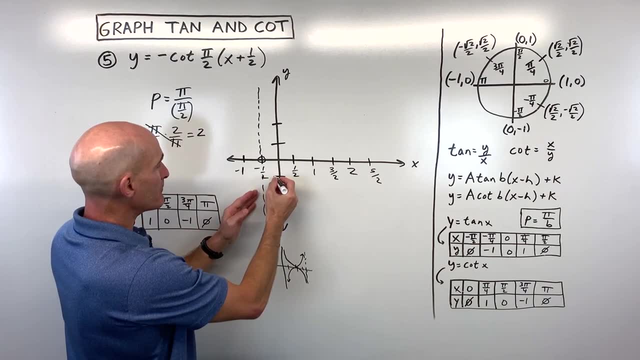 So now, instead of going like this, the graph's actually going to go like this, up to the right. See, it's a reflection over the x-axis. So what I can do is I can say, all right, this is going to be just a value of 1.. 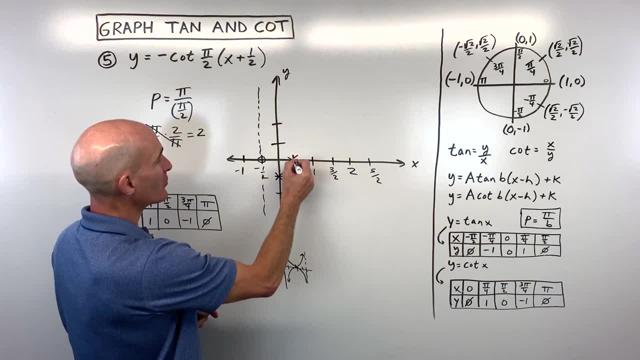 So it's not a stretch or a shrink, It was just a reflection. This is going to go up to the right, And then we're going to have our other vertical asymptote right there, And so this is our, this is our basic cotangent graph that we have here. 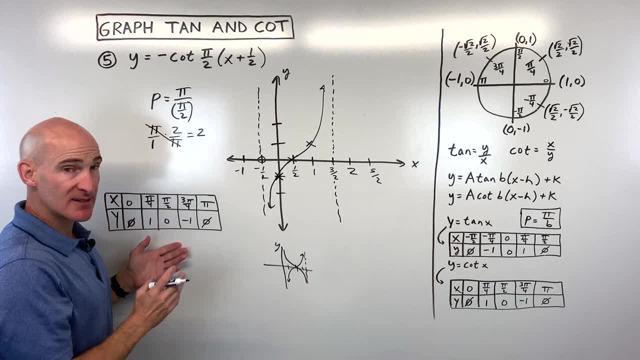 So now you might say, Mario, that was a little tricky, Let's go back to the table method. Okay, so again the table method. you want to memorize these values for cotangent? I just copied that table right here. 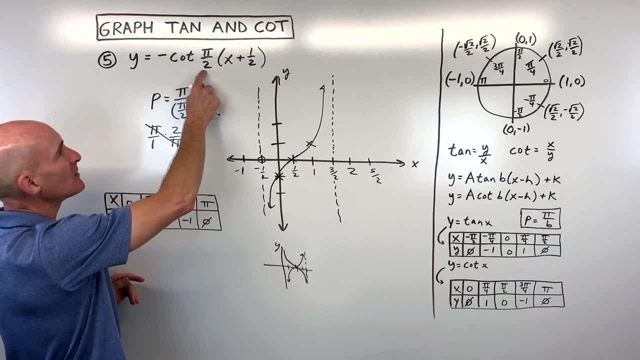 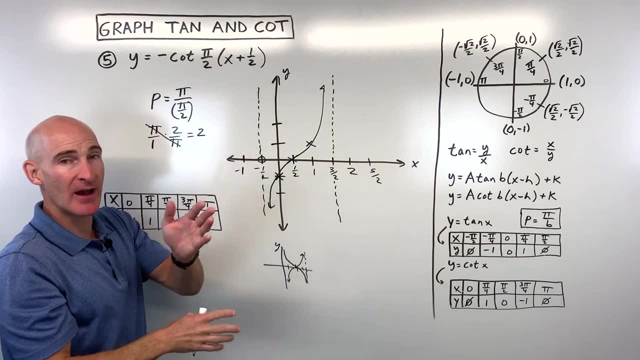 Let's look at the transformation. So pi over 2,. that's going to be affecting the x-values but it has a reciprocal effect. So we're going to multiply everything not by pi over 2, but by 2 over pi. 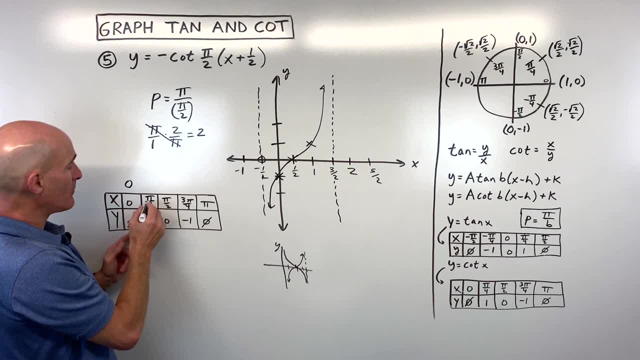 So if I do that, 0 times 2 over pi is still 0.. Pi over 4 times 2 over pi is going to be 1. half Pi over 2 times 2 over pi is going to be 1.. 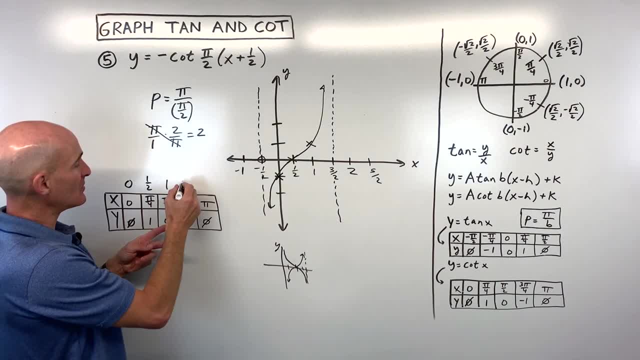 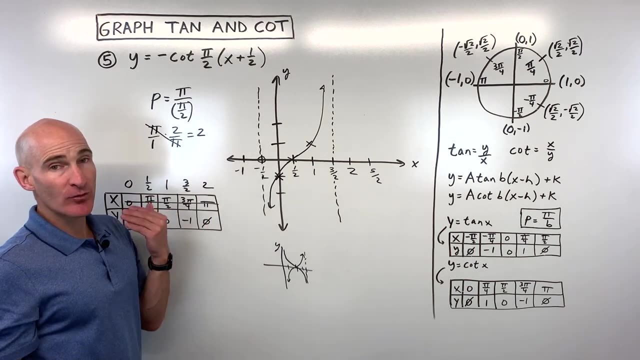 3. pi over 4 times 2 over pi is going to be 3 halves, And pi times 2 over pi is going to be 2.. So let's cross out those old x-values. Now. the plus 1 half is going to shift the graph to the left 1 half. 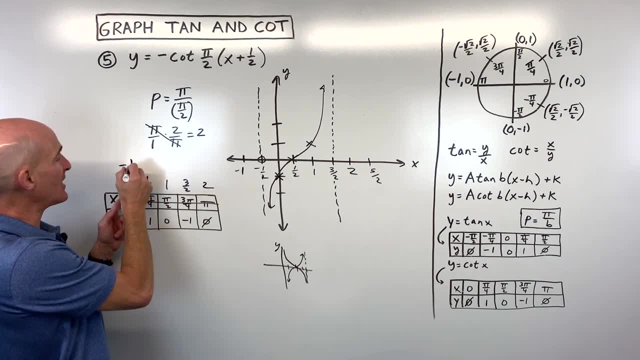 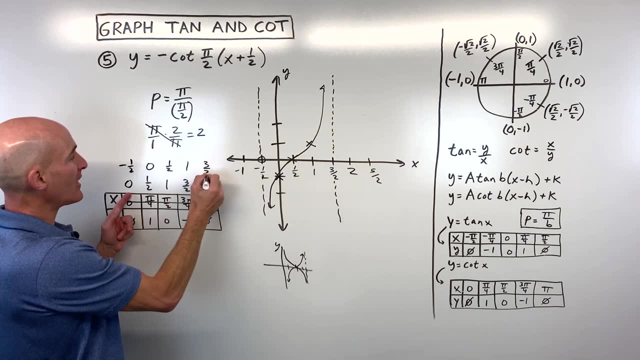 So what I'm going to do is I'm going to subtract 1 half from all the x-values, So that's going to put us at negative 1 half, 0,, 1 half, 1, and 3 halves. Let's cross out those old x-values. 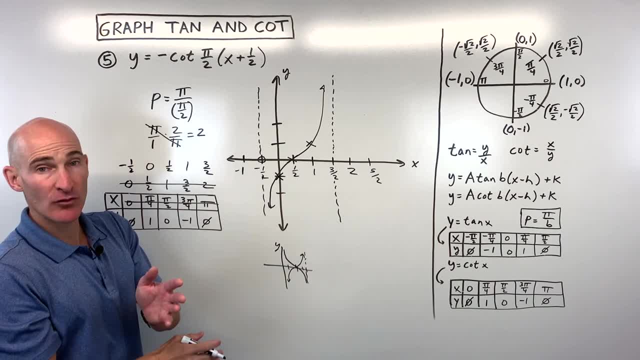 And then this negative we said is going to multiply all the y-values by negative 1.. That's what reflects it over the x-axis. So if I multiply these y-values by negative 1, we're going to get negative 1, 0,. 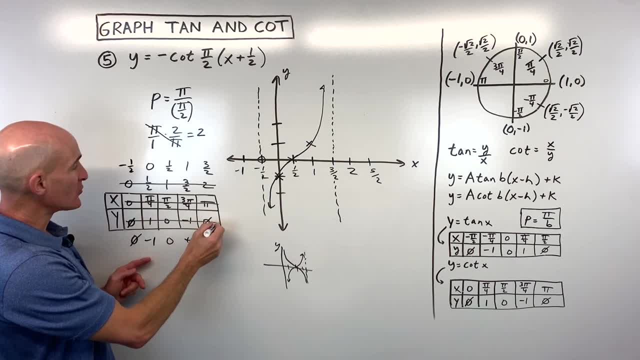 positive 1, and still undefined. So let's cross out those old y-values. So now let's see we've got negative 1, half undefined. so that's where our vertical asymptote is 0,. negative 1,. 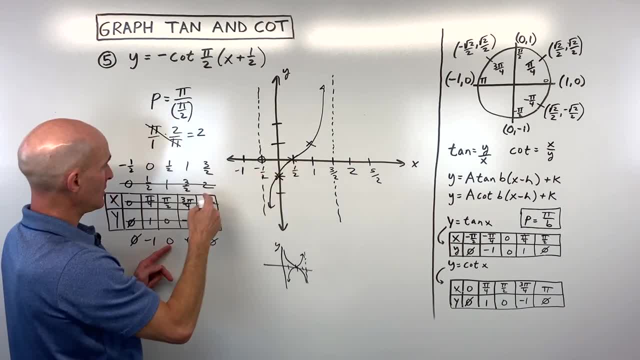 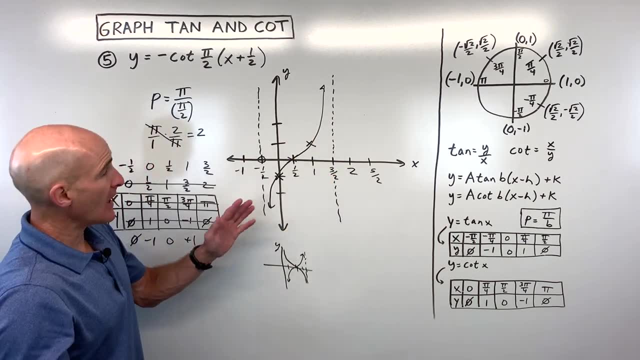 that's this point right here: 1 half 0, 1, 1, and then at 3 halves- undefined- we get another vertical asymptote And again you can repeat that process. So I could say over here, this would be like this: 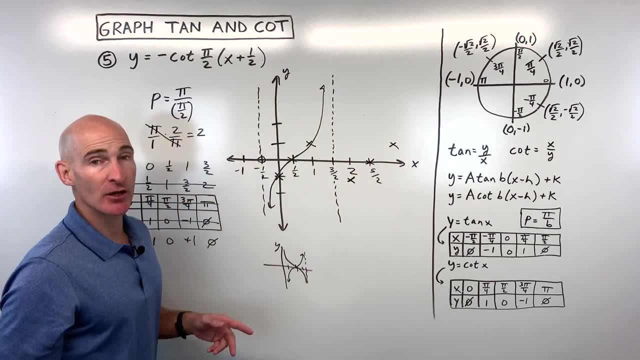 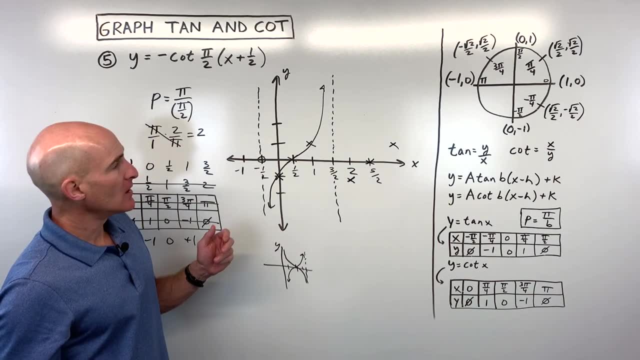 like this, you know, etc. and draw another cycle of our cotangent. Now we haven't talked about domain and range a lot in this video, but let's discuss it a little bit right now. So the domain is really all real numbers. 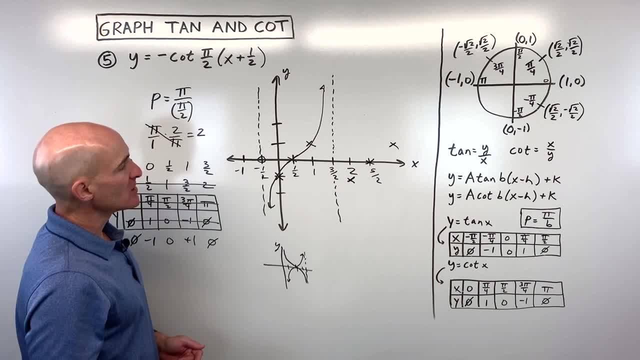 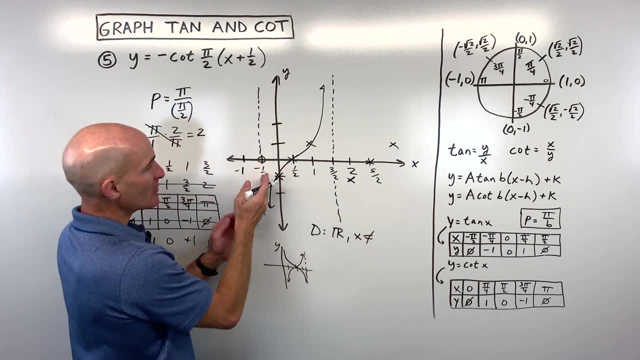 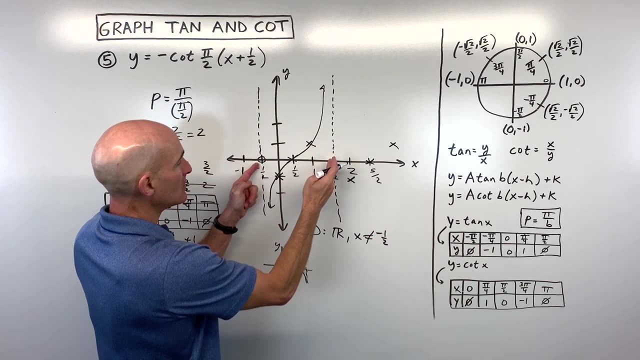 except for where these vertical asymptotes are right. So we could say for our domain: all real numbers, but x cannot equal. now see how this can't be negative 1 half. So it can't be negative 1 half. and then every time we add 2,. 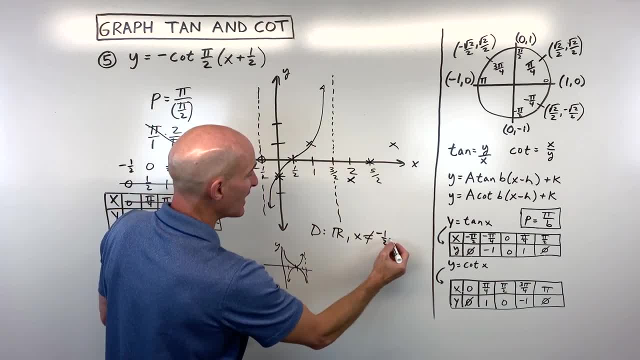 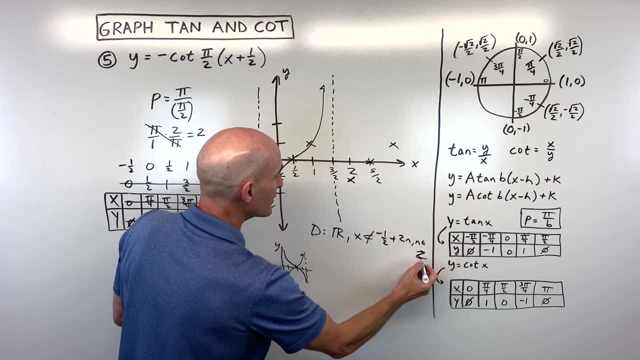 see, because our period was 2, we get another vertical asymptote. So I'm going to say negative 1, half plus 2n, where n is an element of the set of integers, The n can't be like a fraction, like a half or a third. 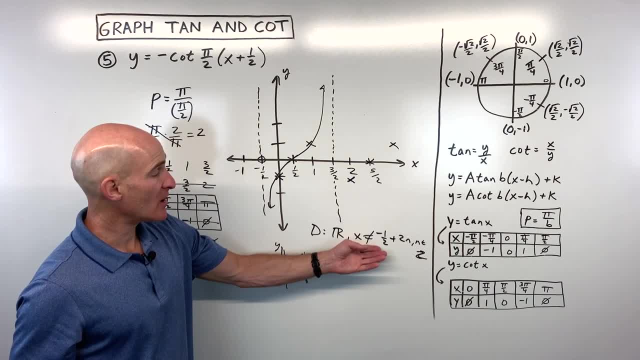 it has to be like 1, 2, 3, or negative 1, negative, 2, negative, 3.. So that would be our domain. But our range- you can see the graph- goes down to negative infinity, up to positive infinity. 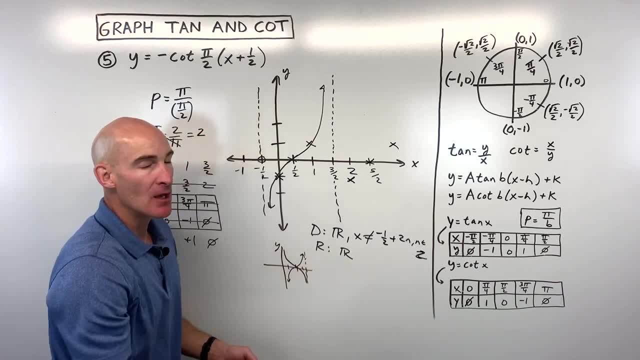 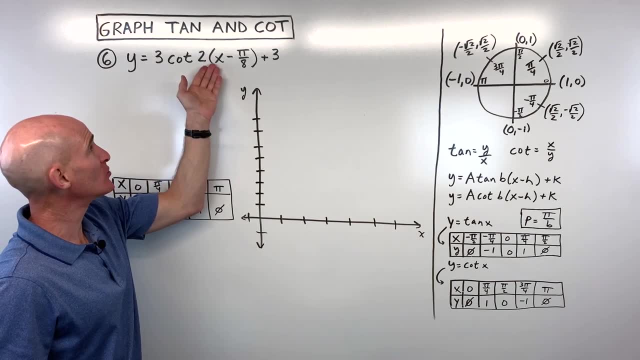 So we would say our range is all real numbers. Let's take a look at another example. Okay, let's look at example number 6. now We've got y equals 3 cotangent 2 times the quantity x minus pi over 8,. 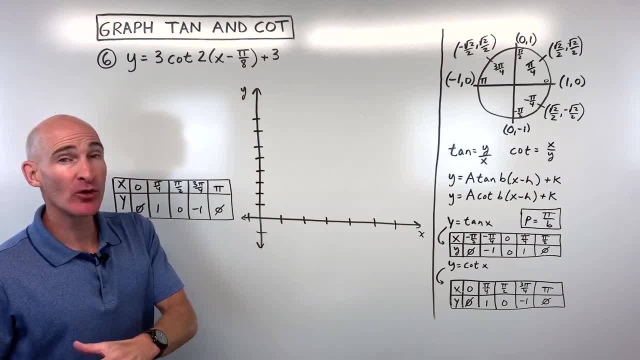 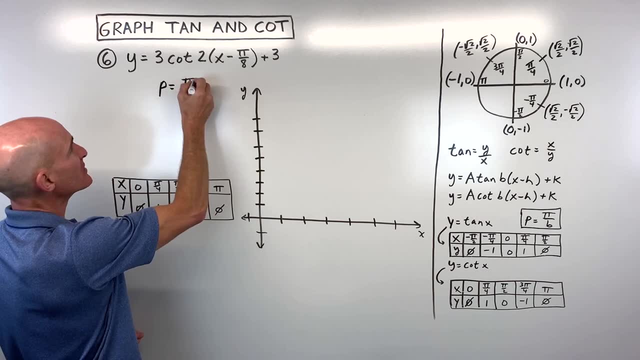 plus 3.. How would we graph that one? Well, let's start with the old school method that I was talking about, that I learned originally- which is to find the period. We know normally that the period for tangent and cotangent is pi. 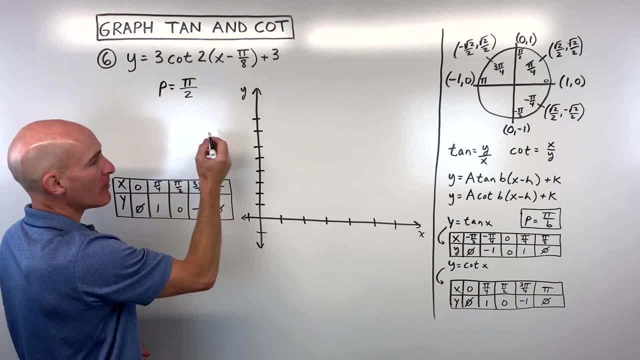 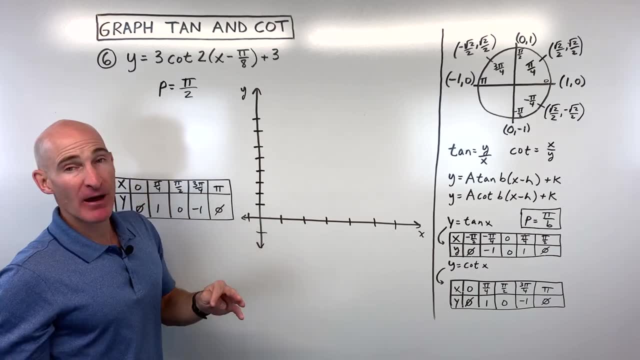 but in this case it's going to be pi divided by b. So pi divided by b is going to give us pi over 2.. Then what I like to do is I like to divide that by 4 or multiply by 1. fourth, 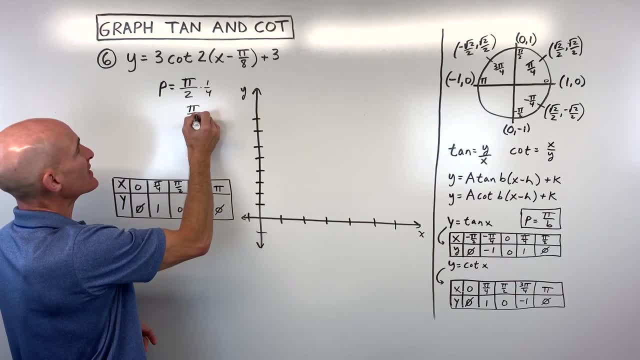 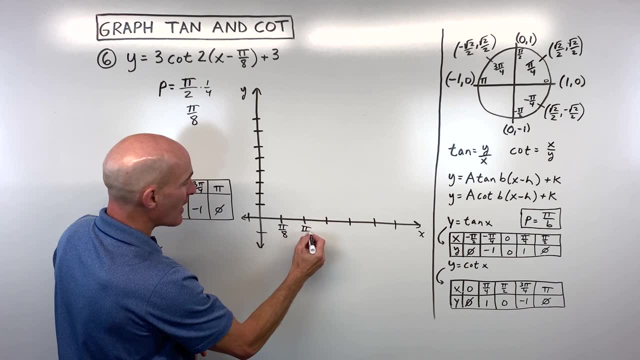 So if I multiply by 1, fourth, that's going to give us a scale of pi over 8.. So on our x-axis, we're going to count, we're going to multiply pi over 8.. So pi over 8, 2 pi over 8, which is pi over 4,. 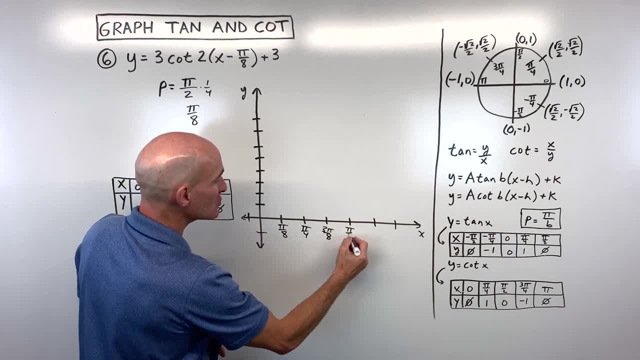 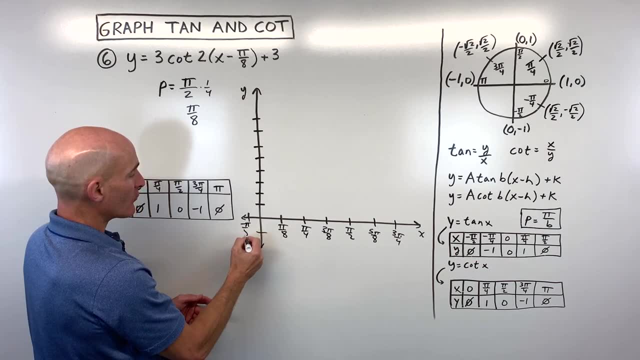 3 pi over 8,, 4 pi over 8,, which is pi over 2,, 5 pi over 8,, 6 pi over 8,, which is 3 pi over 4.. And then you can go the other direction: negative pi over 8.. 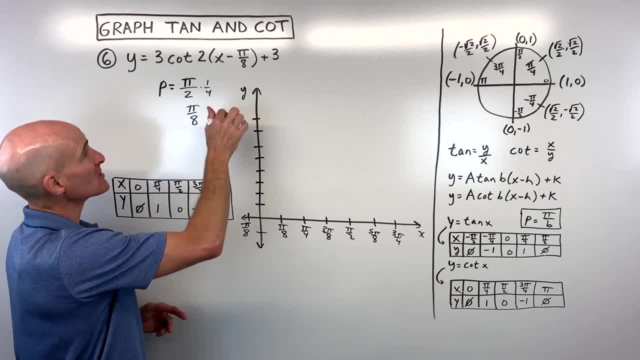 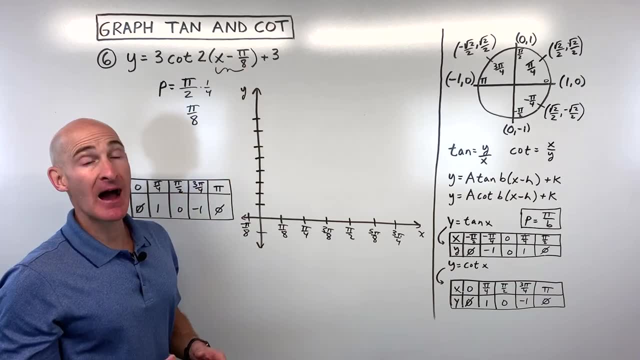 Okay, and then what we're going to do now is we're going to look at the shift. So we're going to say, hmm, what does this minus pi over 8 and this plus 3 do to our graph? Well, remember, whatever is grouped with the x has the opposite effect. 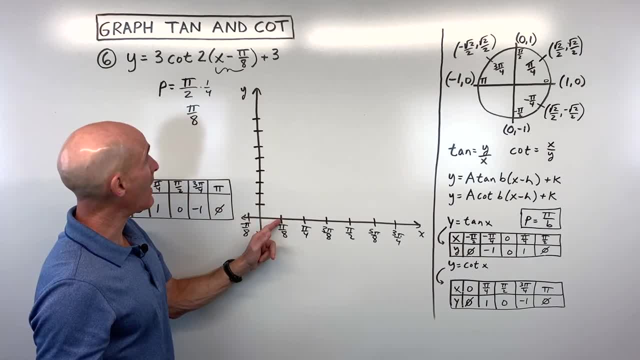 Okay, so the minus pi over 8 is going to actually shift the graph right: pi over 8.. This one has the same effect. It's going to shift it up 3.. So I'm going to think of this point right here. 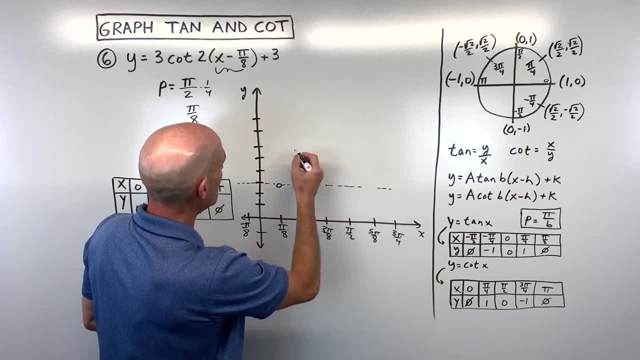 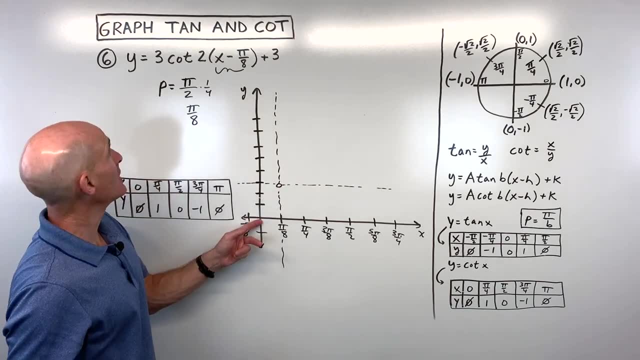 kind of like my new origin, kind of like my new x-axis and kind of like my new y-axis going through this point right here. So it's kind of like our new starting point. Okay, instead of from here, Then what we're going to do is from this point. 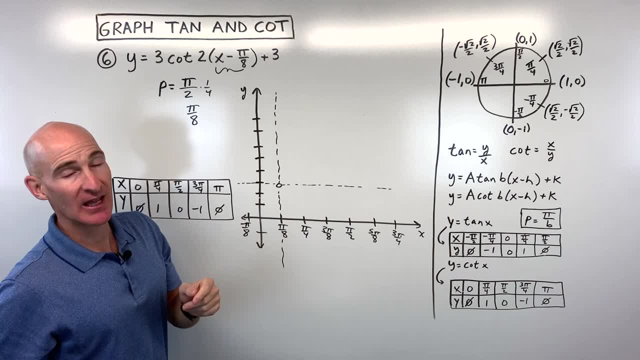 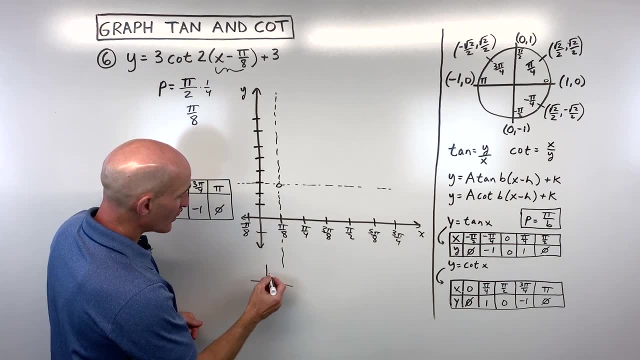 we're going to graph. y equals 3 cotangent. Okay, so the 3 we know is going to have a vertical stretch by a factor of 3.. Now, keeping in mind what cotangent looks like, remember how it looks like this: 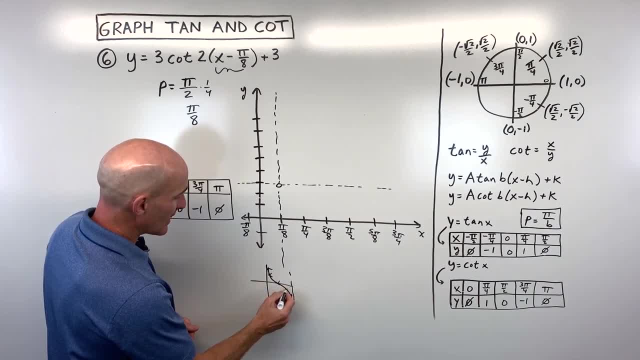 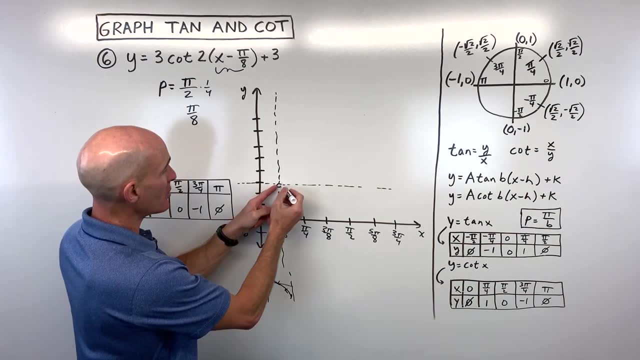 It goes down to the right and it's like that's what our basic graph is. So this point here, which is normally at 1, is going to be at 3 times 1, which is 3.. So from here, when I go right one step up 3, I'm going to have a point right there. 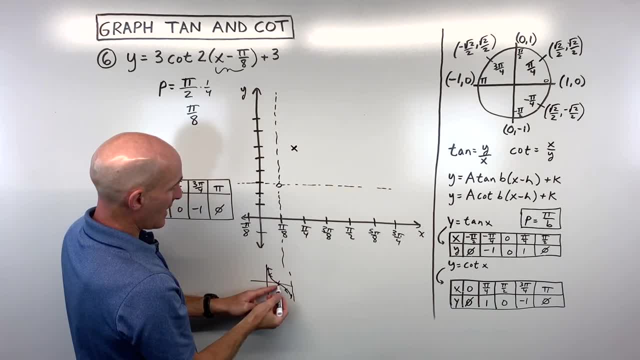 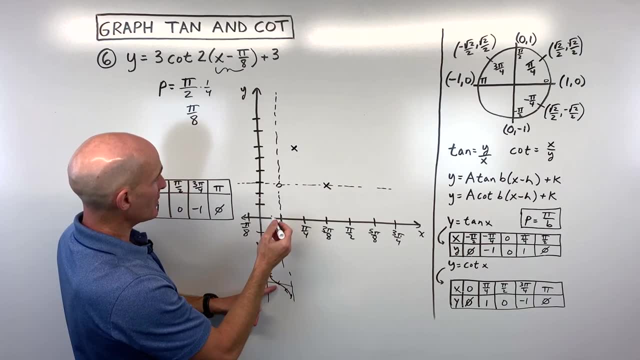 Then here I'm just going to go right through the x-axis, which this is like our new x-axis, so it's going to be right here, And then it's going to go down by 3.. So let's see 1,, 2,, 3, it's going to put us right here. 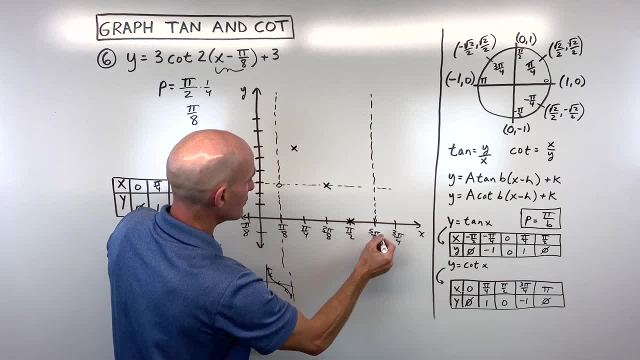 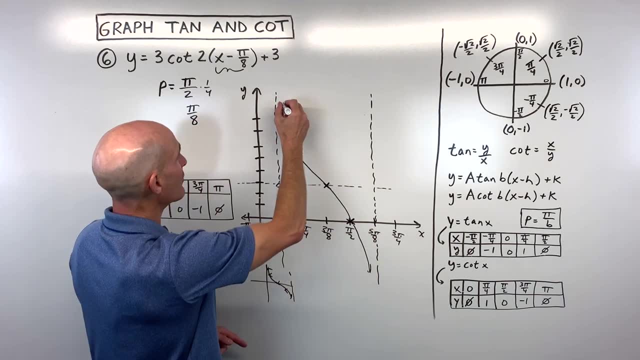 And then the next one. we're going to have our vertical asymptote right here at 5 pi over 8.. Okay, so that's our basic cotangent graph. Now a lot of students might be saying, Mario, that's kind of a tricky way to do it. 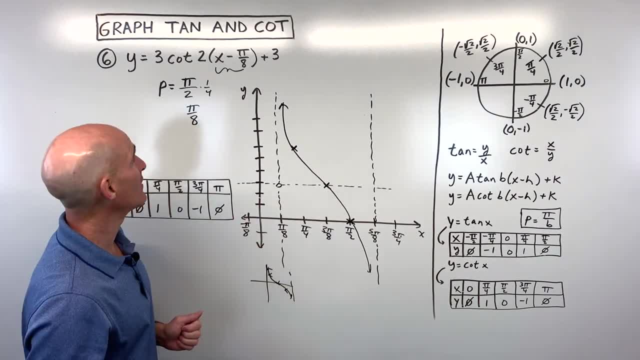 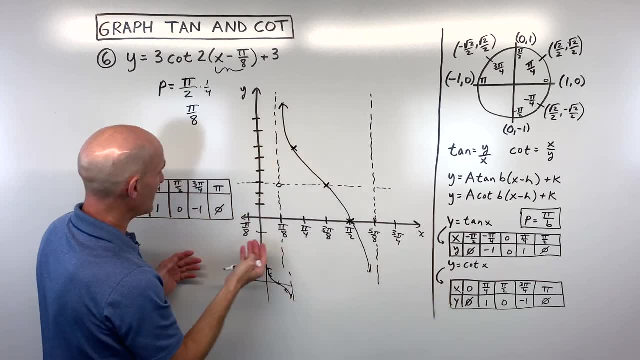 Right, Some students might say, oh, that's a quick way to do it. So, depending on which way you view it, pick that method. So for the other method, let's just go back to our table. Okay, here's our cotangent table. 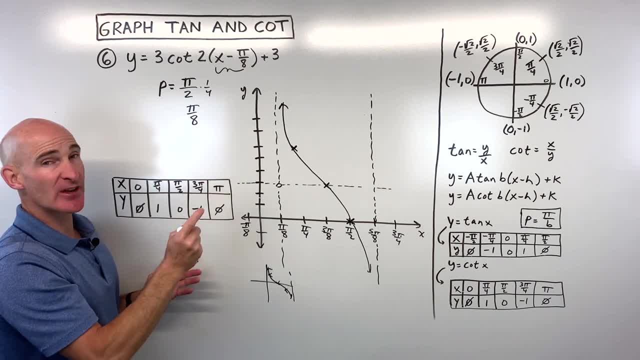 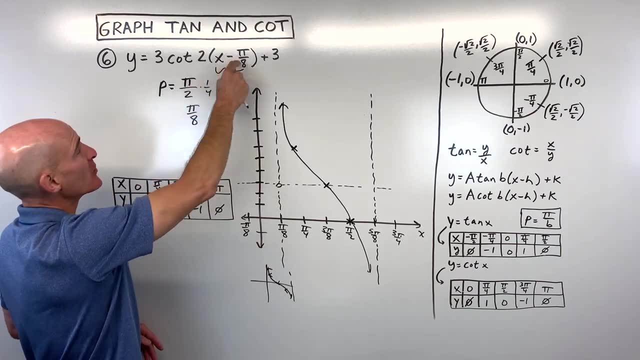 And let's look at the transformation. So the key thing with these transformations is: you want to do this k value last. okay, that's our vertical shift up and down. And then, with these values here, you want to make sure you do the. 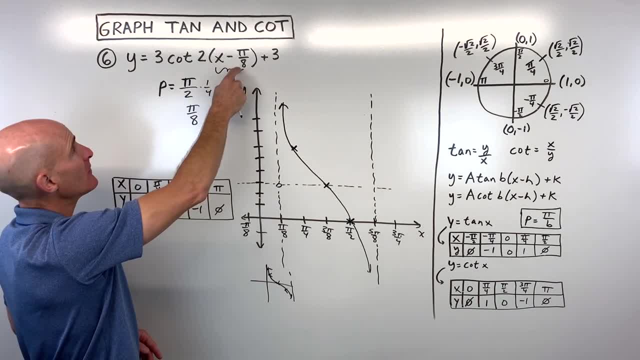 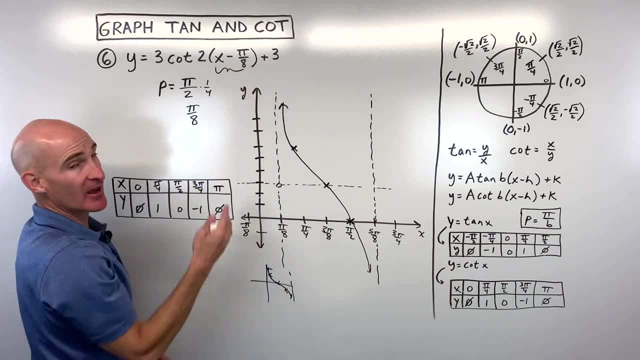 horizontal stretch or shrink and then the shift second, Okay, but if you want to keep a real simple order, when it's in this form like this, you could just do a, b, h, k and you'll get the right graph. 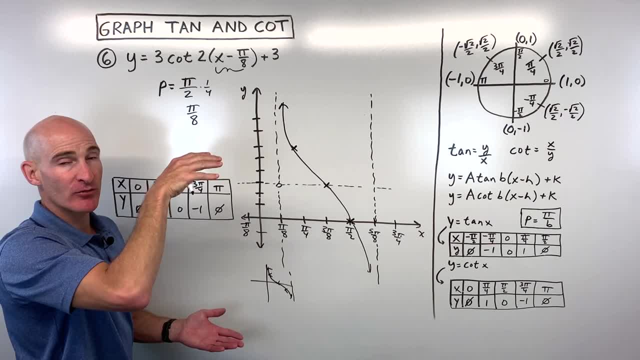 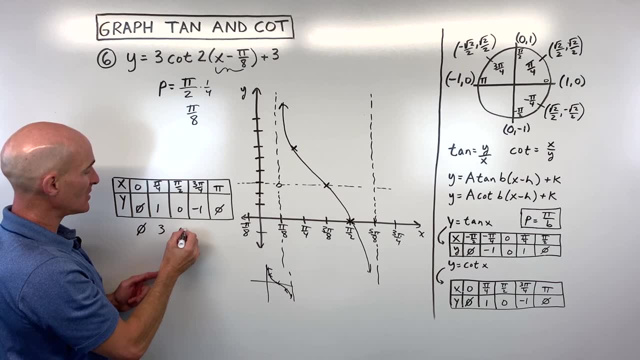 So here we'll do it that way. So the 3 is going to be a vertical stretch by a factor of 3, which means we're going to multiply all these y values by 3.. Undefined times 3 is still undefined. 1 times 3,. 0 times 3, negative 1 times 3, undefined times 3.. 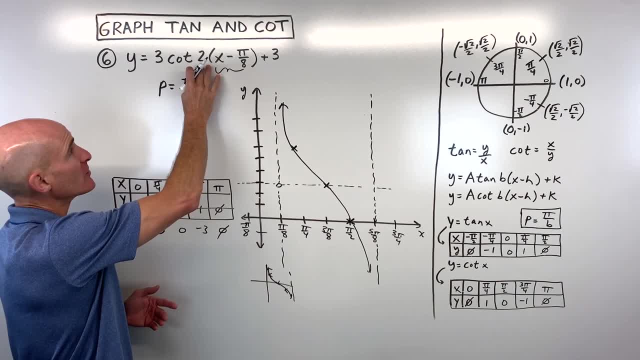 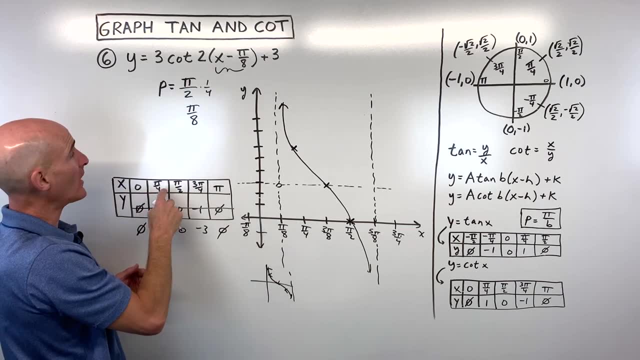 Cross out the old y values. Okay then, going to the b value, the 2,. whatever is grouped with the x has the reciprocal effect, which means we're going to multiply all the x values not by 2, but by 1 half. 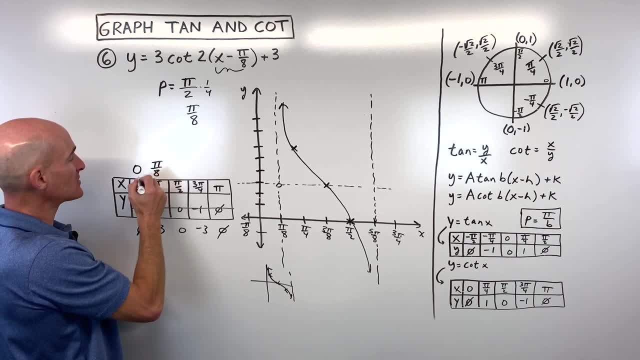 So 0 times 1 half is 0.. Pi over 4 times 1 half is pi over 8.. Pi over 2 times 1 half is pi over 4.. Pi over 4 times 1 half is 3 pi over 8.. 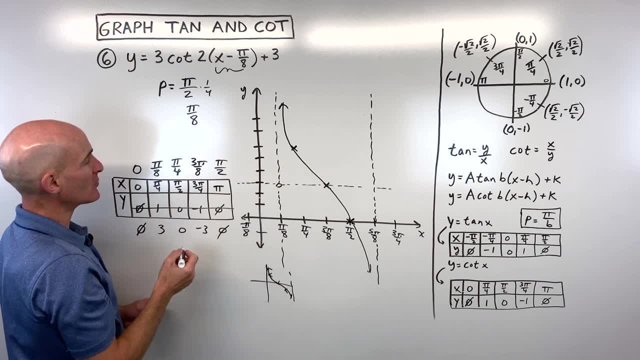 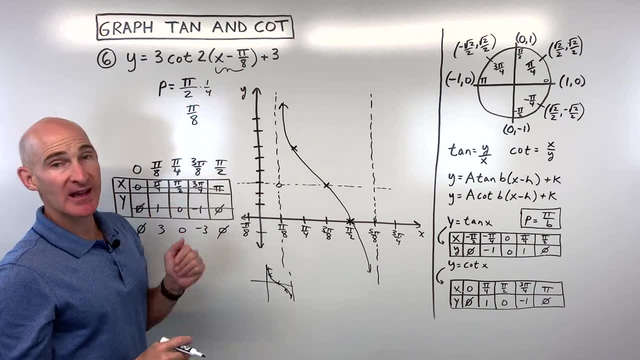 And pi times 1 half is 4, pi over 8 or pi over 2.. Cross out the old x values, Then going to the h value, the minus pi over 8, again it's grouped with the x. It has the opposite effect. 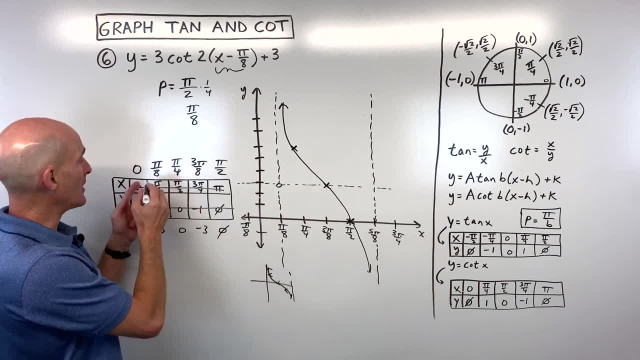 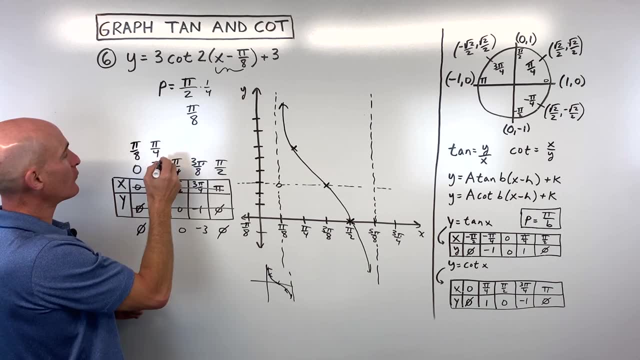 It's going to actually add pi over 8 or shift the graph right: pi over 8.. So if we do that, add pi over 8 to all of our x values, this is going to be pi over 8,, 2 pi over 8, which is pi over 4,. 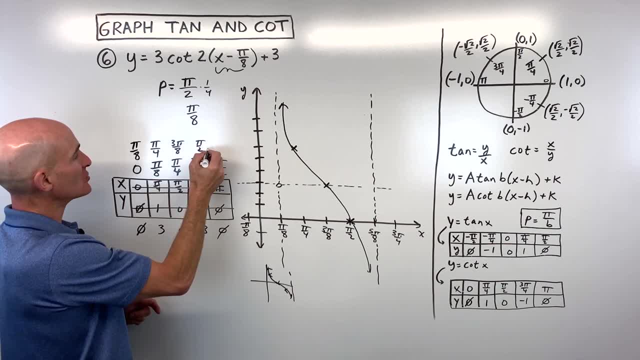 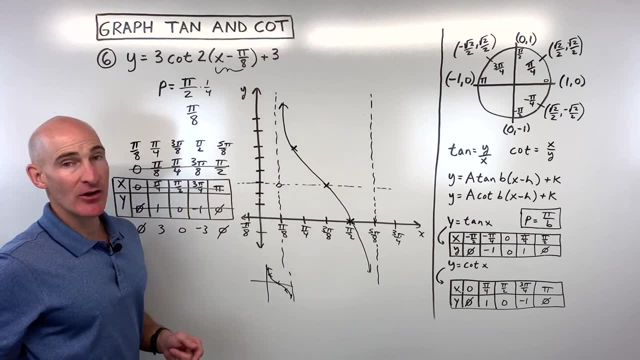 4 pi over 8,, 4 pi over 8,, which is pi over 2,, 5, pi over 8.. Cross out those old x values. And then, lastly, this plus 3,. this k value is going to shift the graph up 3,. 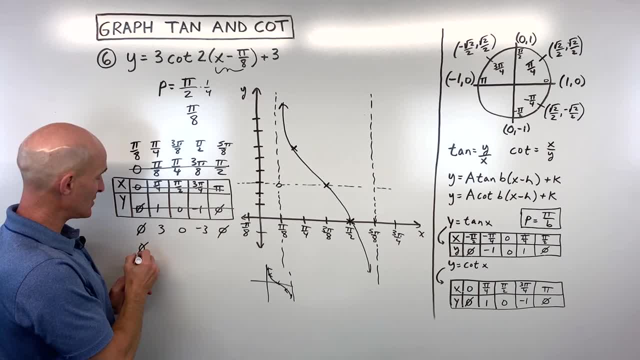 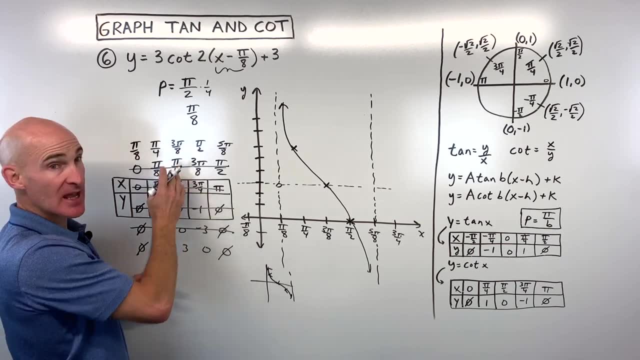 which means we're going to be adding 3 to the y values Undefined, plus 3 is still undefined. 6, 3, 0, undefined. So now we've got our table, Let's check it. So we've got pi over 8, undefined. 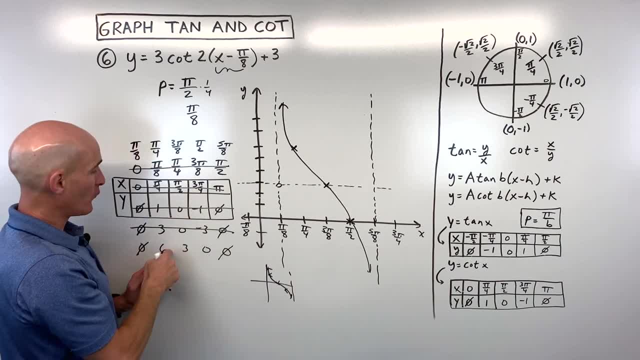 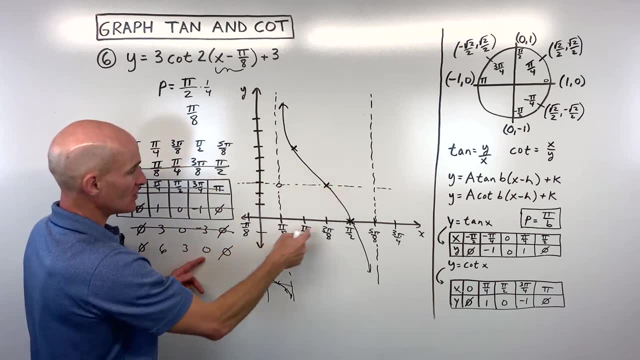 So pi over 8, undefined vertical asymptote, Pi over 4. We're at 6.. OK, perfect 3. pi over 8 is 3.. OK, good, Pi over 2 is 0.. That's right on the x axis. 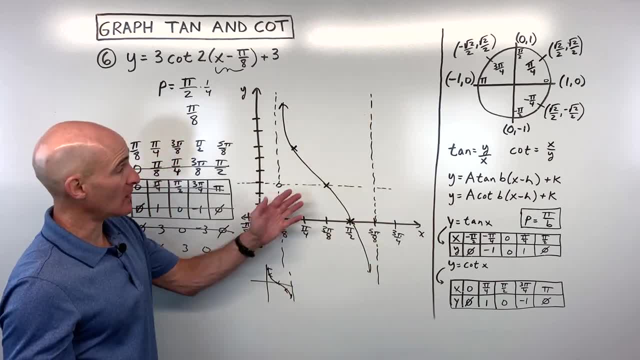 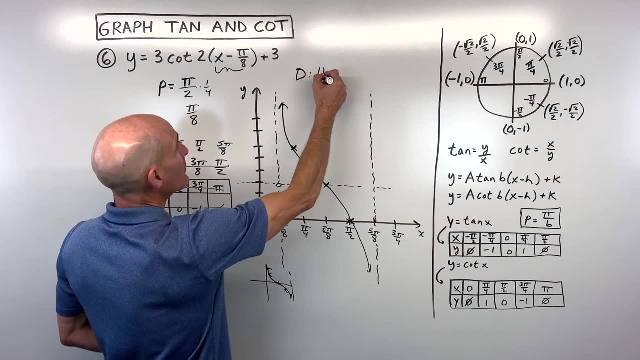 5 pi over 8- undefined- We get another vertical asymptote And that's one period or one cycle of our graph. If we want to ask ourselves what's the domain, We know it's going to be all real numbers, except for x, cannot be where the asymptotes are. 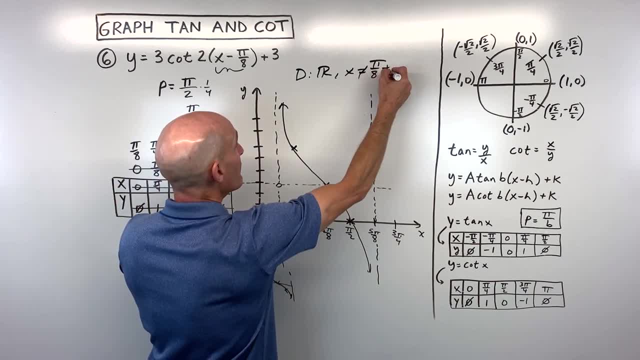 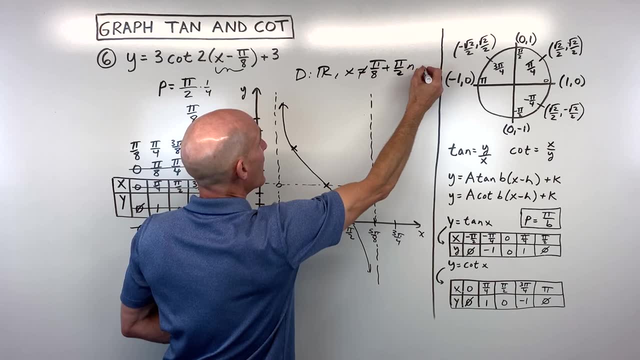 Now their first asymptote here looks like it's at pi over 8.. Plus we keep adding one period which is pi over 2.. So we're going to say plus pi over 2n, where n is an element of the set of integers. 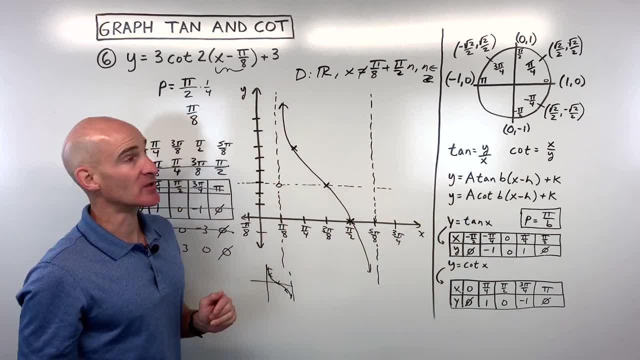 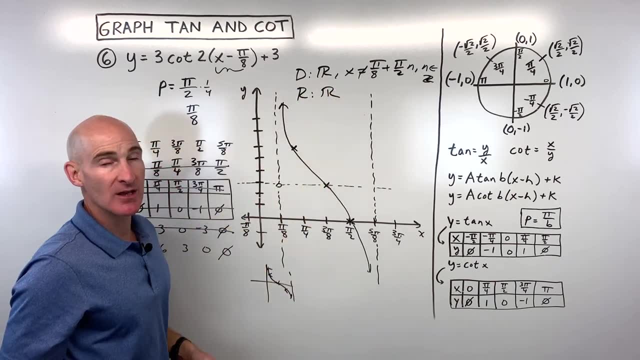 Meaning, every time we add pi over 2, we get the next vertical asymptote, next one, next one, etc. The range, though you can see, it's going up and down forever and ever. So the range is going to be all real numbers. 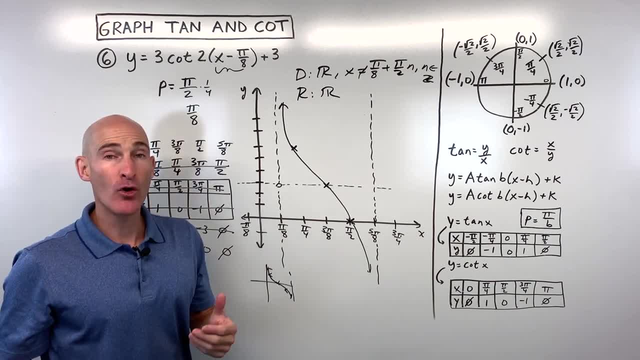 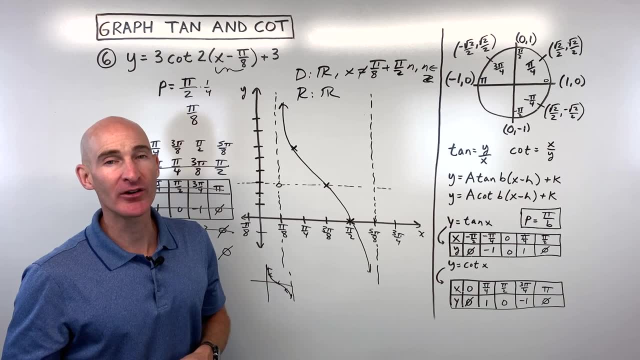 Now let's take a look at two more examples, And I encourage you to practice these on your own. We're going to do one tangent graph, one cotangent graph. Use whichever method you feel that you like best, and we'll go over them together. 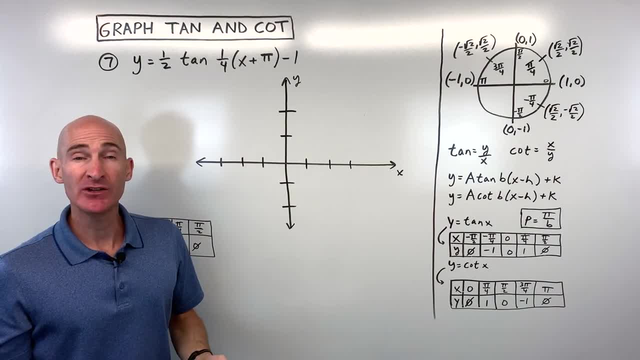 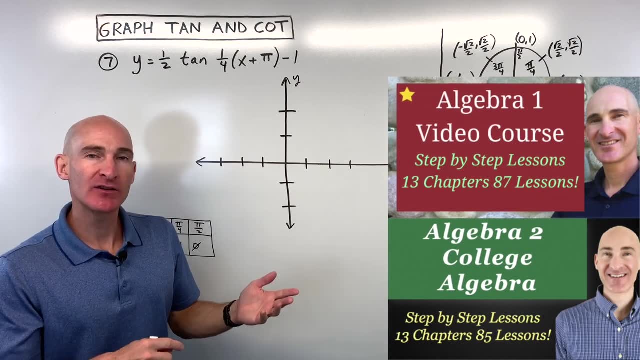 If you like the way that I explain things and you want to go deeper into Algebra 1 or Algebra 2, slash college algebra, check out my video courses for sale. I'll put a link in the description below. Both video courses have about 85, 87 lessons or so. 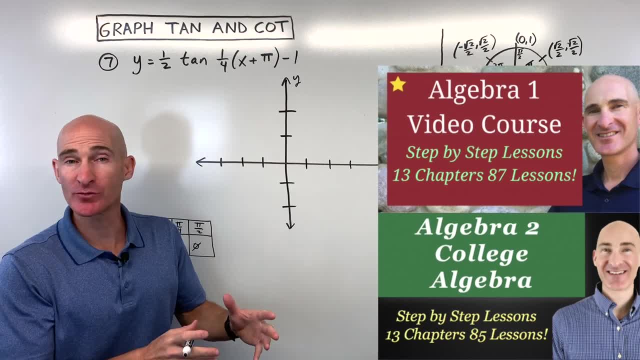 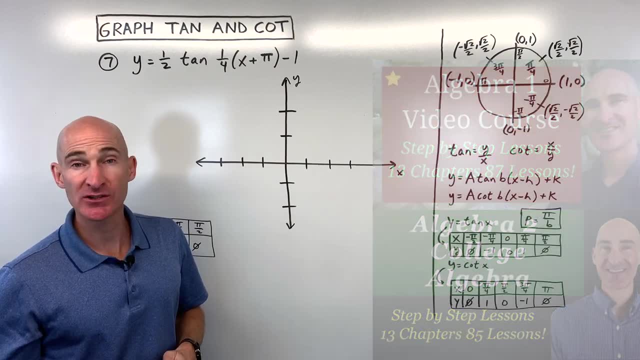 And I walk you through a typical curriculum: Algebra 1 or Algebra 2, slash college algebra, building on each previous concept. So great resources there if you're studying those classes or want to review, And if you just want to support the videos that I'm putting up here on my Myers Math Tutoring YouTube channel. 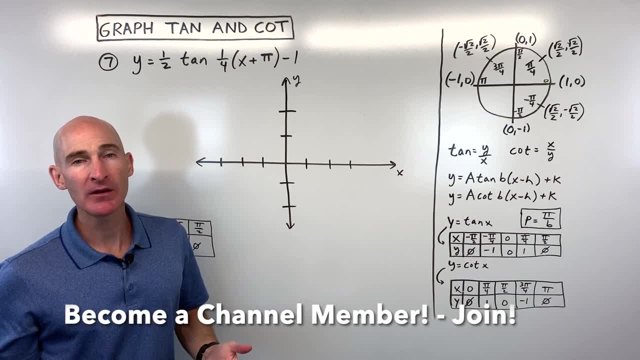 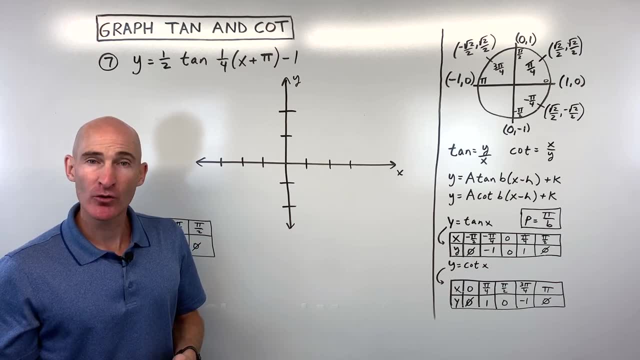 consider becoming a channel member. So for a few dollars a month you can be a supporter of the channel And I really appreciate that. And lastly, if you just want to find another way to support me, you can check out my Teespring store where I sell some fun math T-shirts. 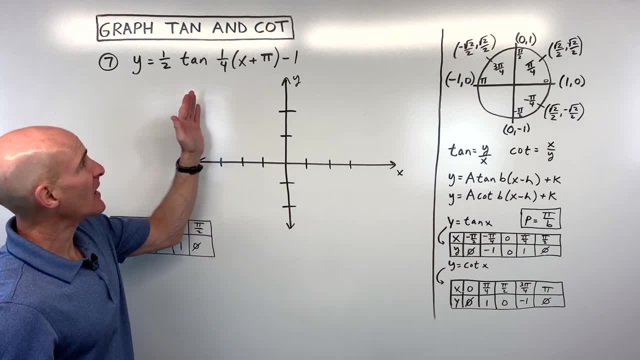 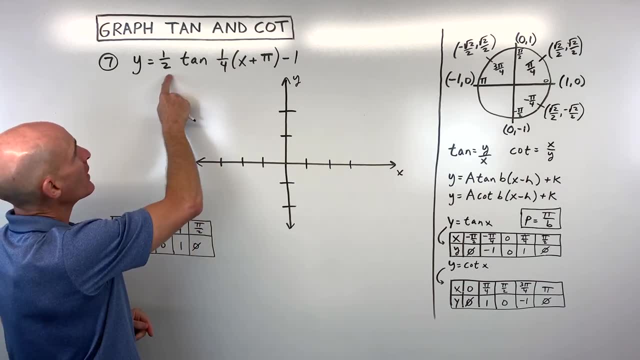 So you can see those links in the description as well. But let's dive into this last couple examples where you get some chance to practice graphing tangent and cotangent. First graph this tangent, graph One, half tangent one. fourth: x plus pi minus one. 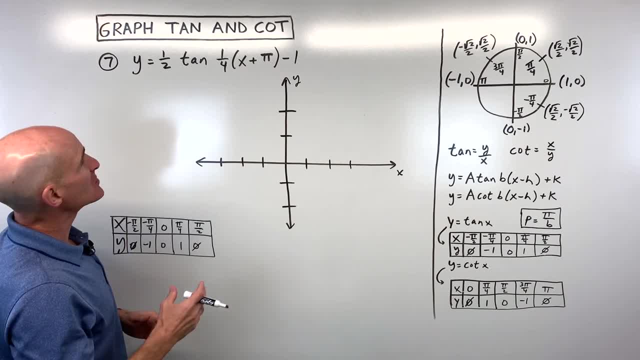 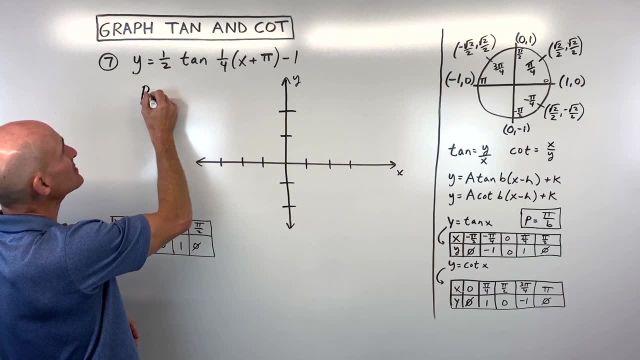 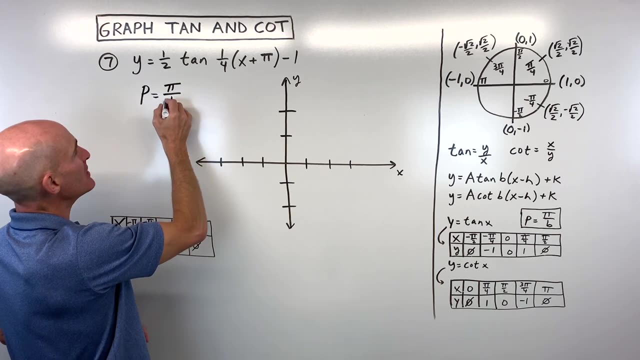 How would you do that one? Go ahead and pause the video. Now, if I was going to do this, I'm going to show you the two methods. One method I learned originally back in high school from my excellent teachers was to start with this b value. so period is equal to pi divided by b. 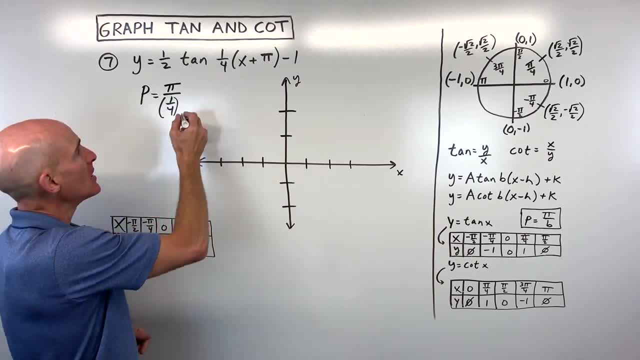 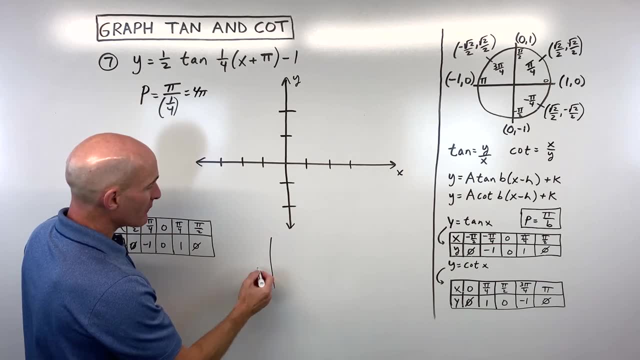 So pi divided by one fourth. When you divide by a fraction, you multiply by the reciprocal, And so that's going to give us a period of four pi. Now remember our basic shape, for tangent looks something like this: Remember how half the graph was on the left side of the y axis and half was on the right. 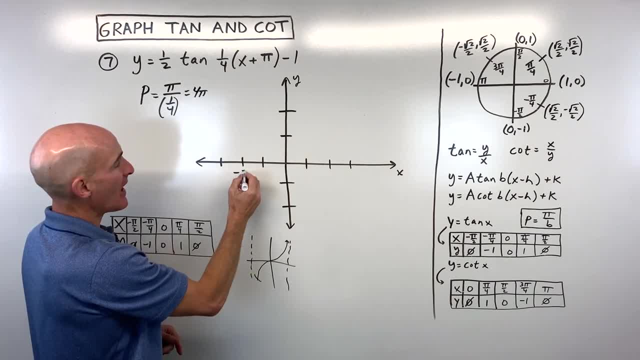 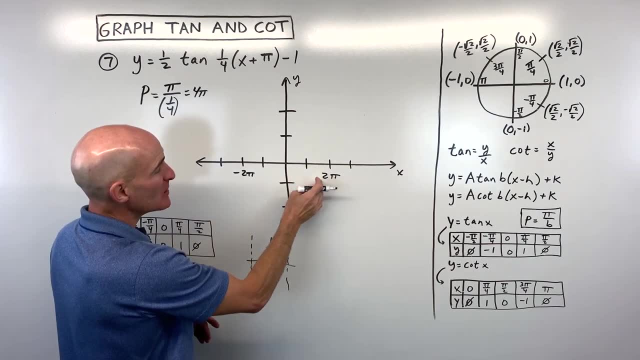 And so what I'm going to do is I'm going to take this four pi and I'm going to cut it in half: Negative two pi and positive two pi. That gives me a period of four pi. Then I'm going to find these midway points. 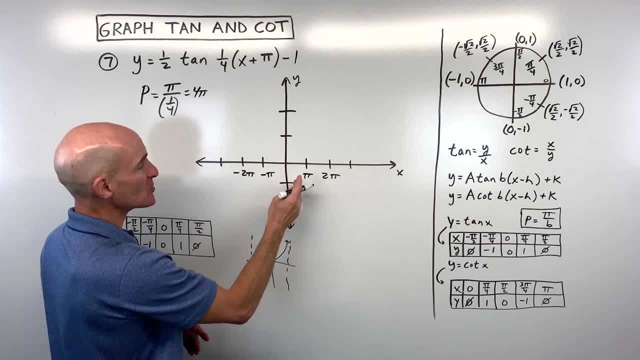 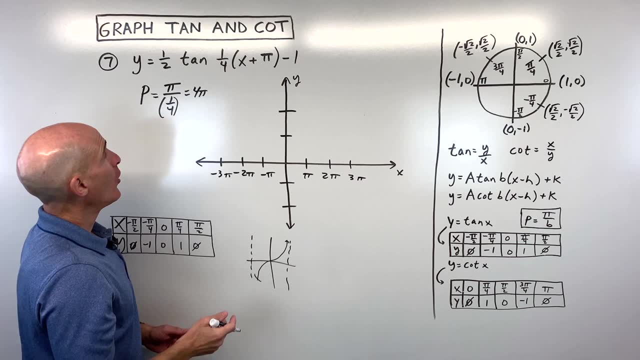 Halfway of two pi is one pi, and this would be negative pi. So you can see that our scale is pi. We're counting by pi at each one of these Intervals. OK, then what I would do is I'd look at the shift. 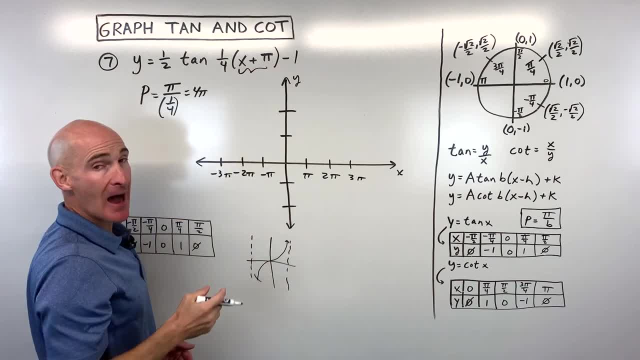 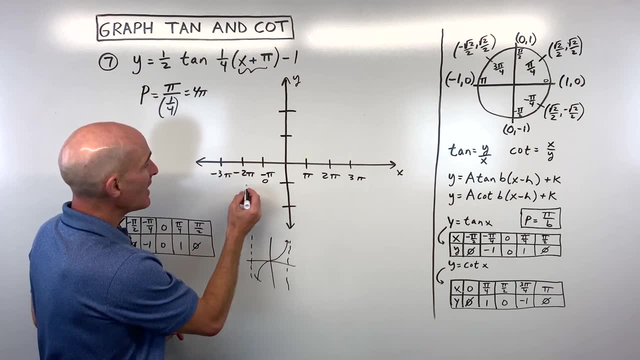 I'd say: plus pi, minus one, whatever is group of the x has the opposite effect, right. So the plus pi is going to shift left pi and the minus one is going to go down one. So I'm going to think of this as like our new x axis, our new y axis. 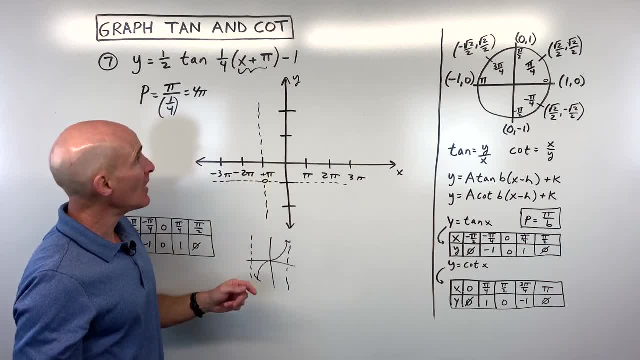 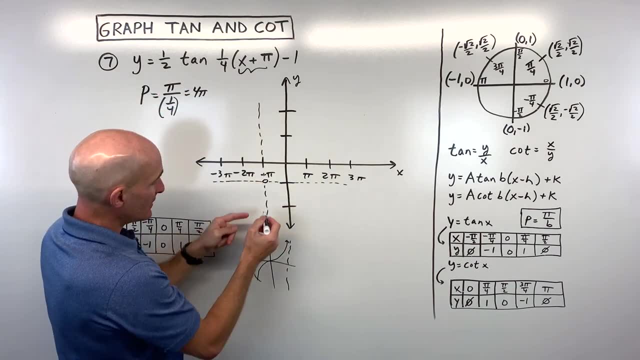 Essentially this is like our new origin And I'm going to graph from here our tangent graph, but with a vertical shrink of one half. So normally with tangent it goes right through the origin. This is like our new origin, right here. 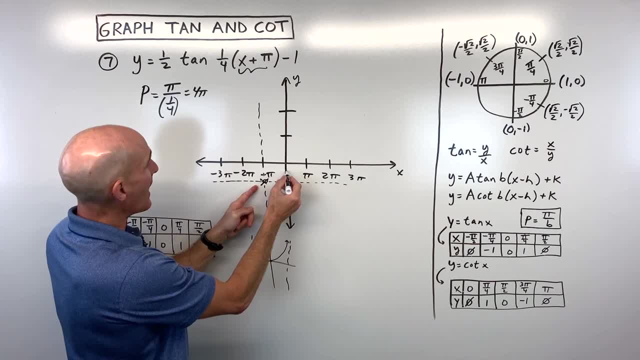 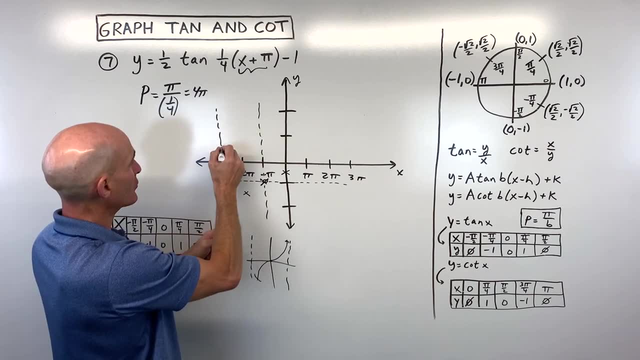 But then when I go over one step, I'm going to go up a half, And when I go left one step, I'm going to go down a half. OK, and then I have my vertical asymptote here and my other vertical asymptote here. 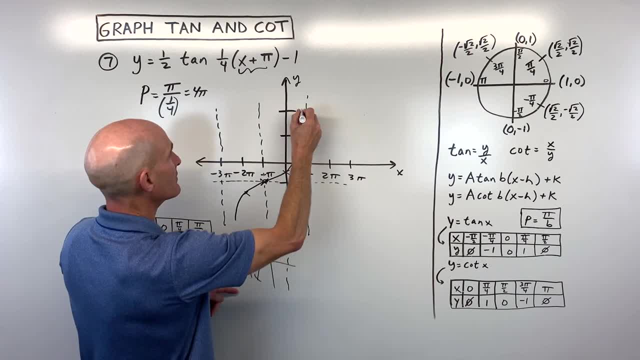 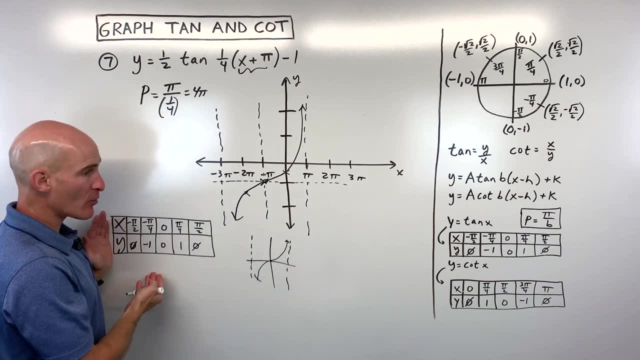 And so our basic graph here is going to look something like this and it's going to repeat. Now, if you don't like that method, let's look at the table method. So, again, you want to memorize these values for tangent. 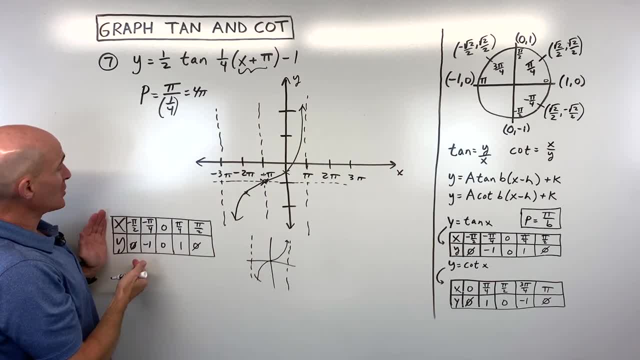 Again, if you forget, you can go to your unit circle And then what we're going to do is we're just going to do a, b, h and k, So the one half is going to multiply all the y values by one half. 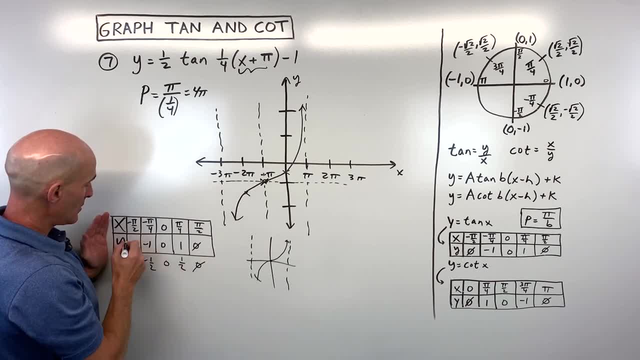 So let's go ahead and do that. Cross out the old y values, The b, the one fourth is going to multiply all the x values by the reciprocal by four. So if we do that that's going to give us negative two pi. 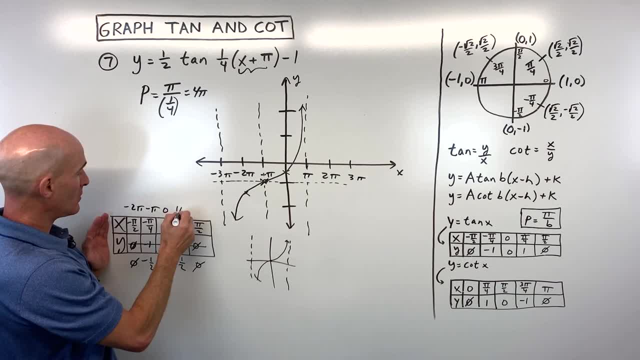 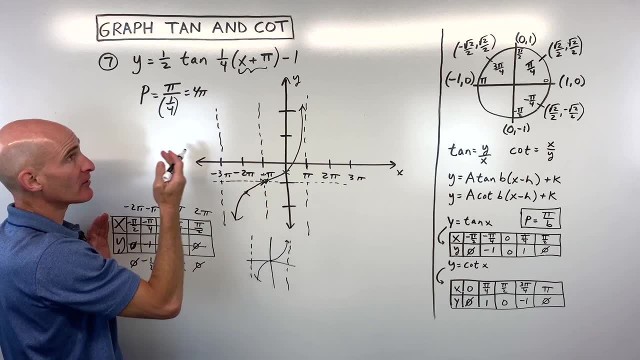 Let's see Negative pi, zero pi and two pi Cross out the old x values. The h is going to shift the graph left pi because, remember, this has the opposite effect. So we're going to subtract pi from each one of these x values. 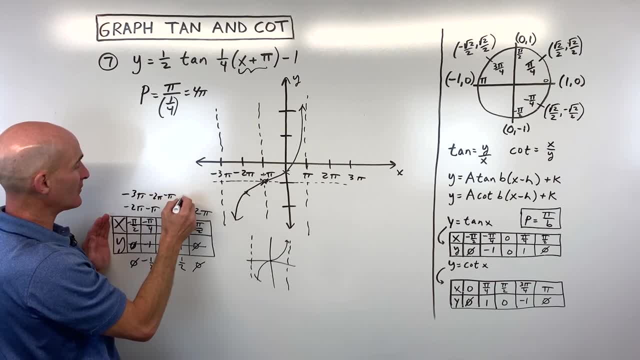 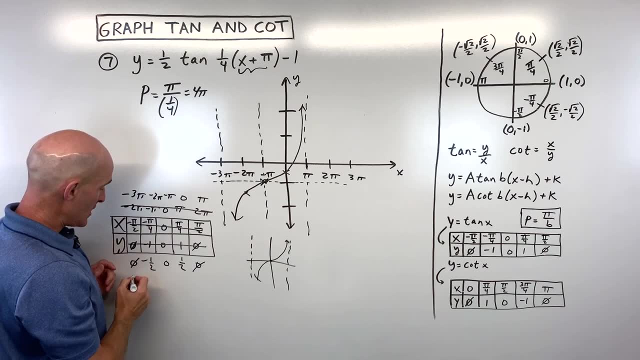 So that'd be negative. three pi negative, two pi negative, pi zero and pi Cross out the old x values. And then the minus one is going to shift the graph down one. So we're going to subtract one from each of these y values. 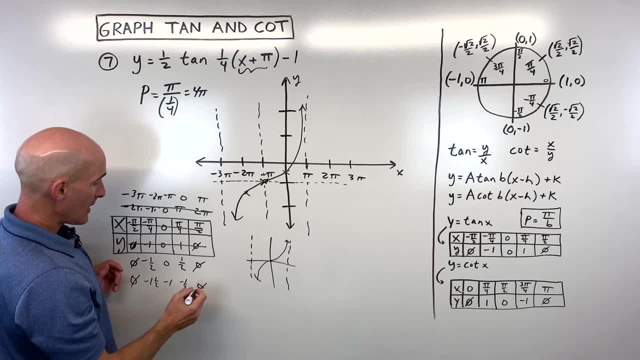 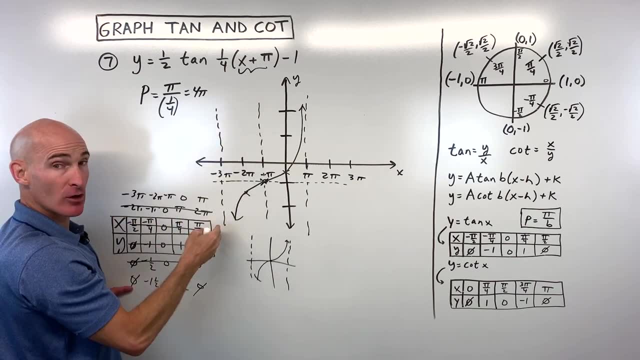 And cross out the old y values. So now we can plot our points. Negative three pi is going to be undefined. So you can see that's where our vertical asymptote is. Negative two pi. we're at negative one and a half. 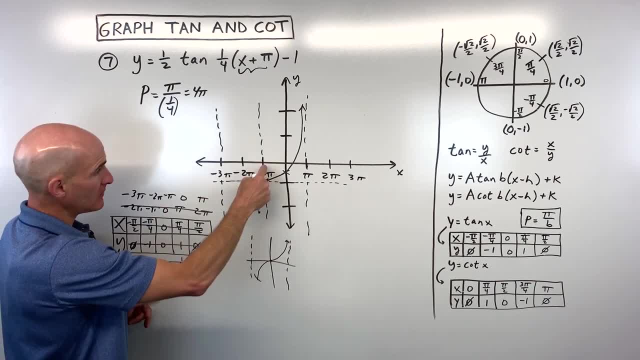 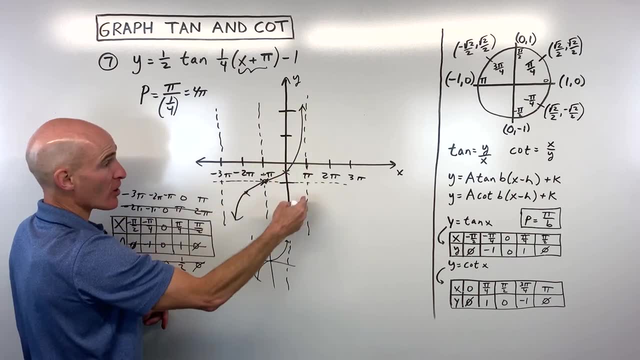 OK, that matches Negative pi. we're at negative one, OK, good. Zero. we're at negative a half- OK, excellent. And then pi we're at undefined. That's where our other vertical asymptote is. So we have a good sketch of our graph. 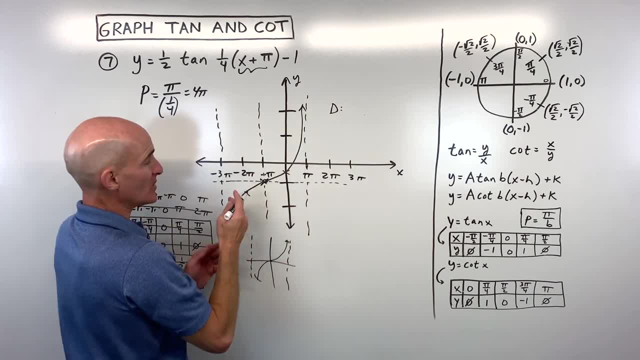 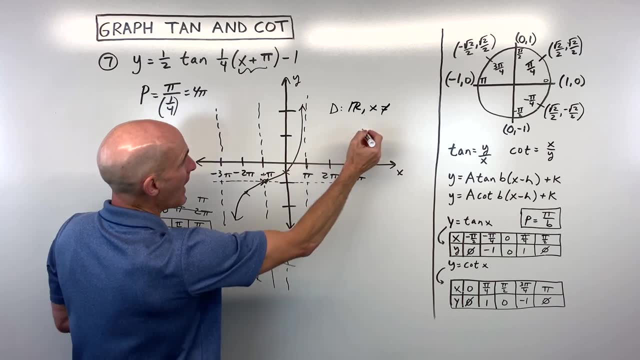 The only other thing you might want to write down here is our domain and range. Domain is all real numbers, but x cannot be. Let's see. let's maybe start with pi. That's a vertical asymptote here and it repeats every four pi. 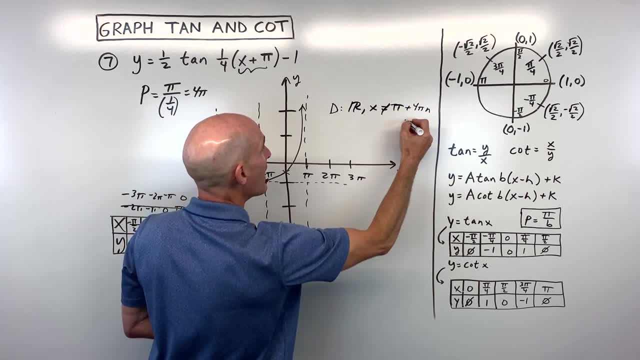 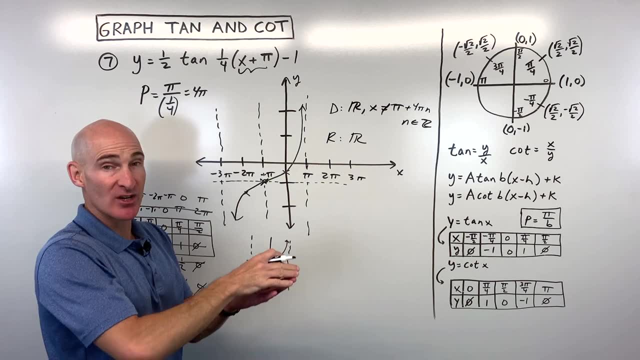 So x cannot be pi plus four pi n, where n is an element of the set of integers. The range, though you can see, for tangent and cotangent, the range is always all real numbers. Let's take a look at one last example. 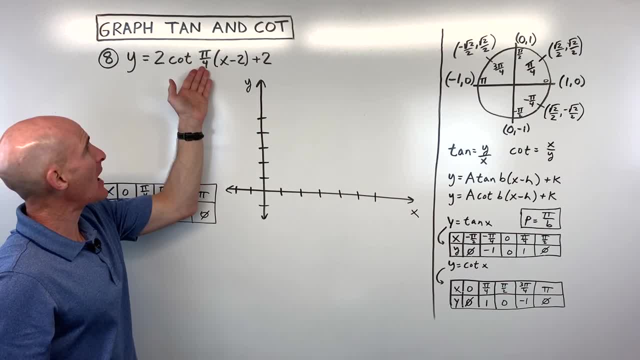 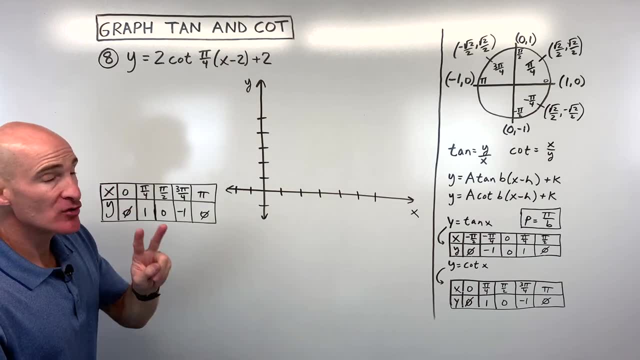 Try this last example: Y equals two cotangent pi over four times the quantity x minus two plus two. How would you graph that? Well, if I was going to do this one, we're going to do the two methods. Let's start by just doing the original method that I learned. 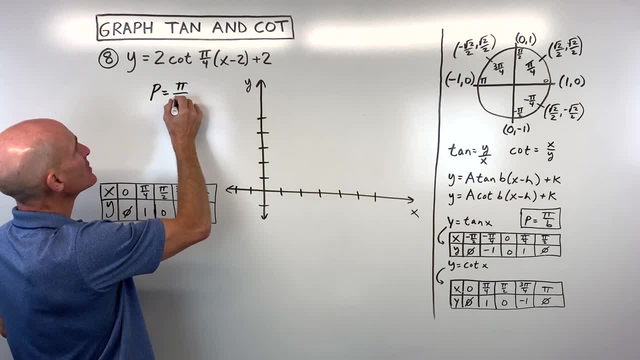 which is the pi divided by b, to find the period. So if we take pi divided by our b value, pi over four, that's going to give us a period of four. Remember, when you divide by a fraction it's like multiplying by the reciprocal. 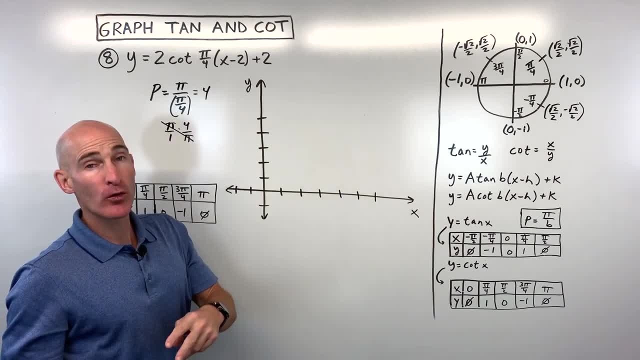 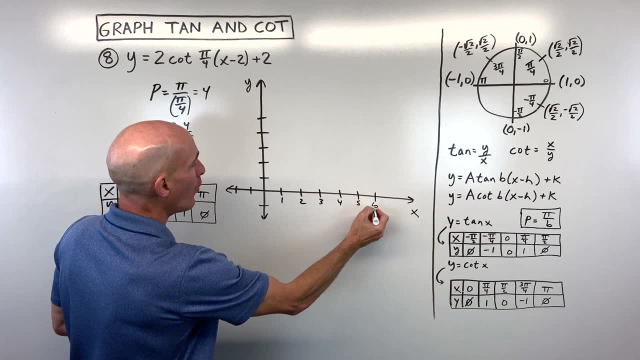 And so then what I would do is I would take that four and I'd multiply by one fourth, or you could divide by four and that's going to give us one. So that means our scale on the x-axis, we're going to be counting by ones. 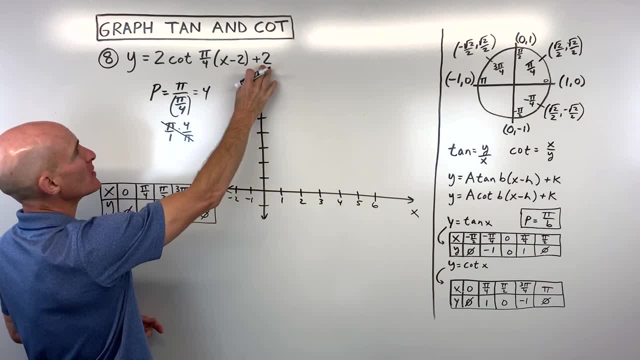 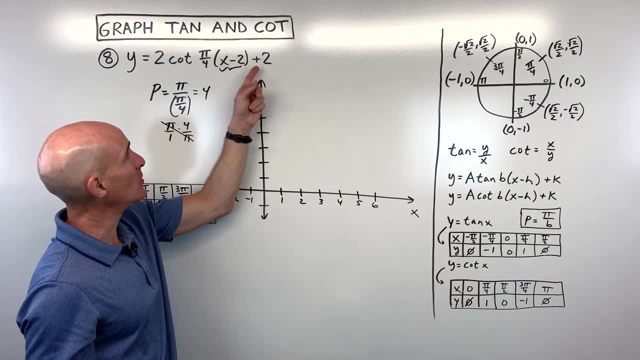 OK, now what we can do is we can look at our shift. So the minus two and the plus two, whatever is grouped with the x, we know, has the opposite effect. So the minus two is going to shift the graph right to positive two. 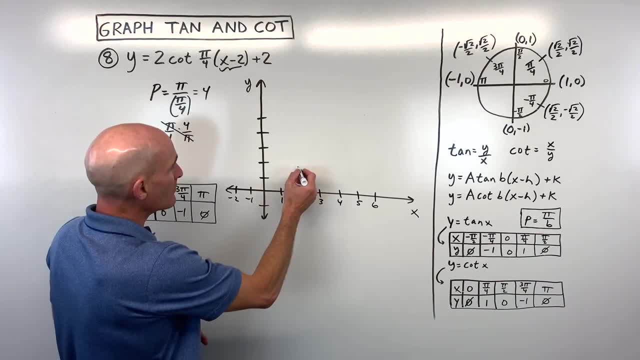 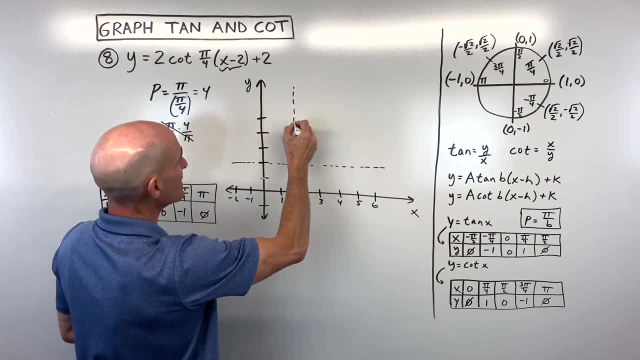 And the k value has the same effect: up two. So right, two up two. we're going to think of this as our new origin, kind of like our new starting point. This is kind of like our new x-axis, kind of like our new y-axis, right. 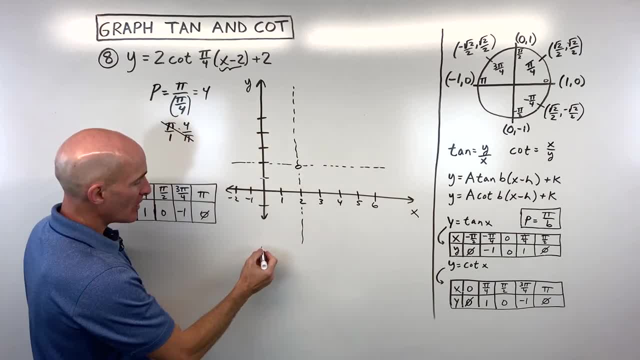 And then the two is going to be a vertical stretch by a factor of two. Now it's good to keep in mind the basic shape of your cotangent graph. So it looks something like this, where it goes down to the right and it has its vertical asymptote right here at the y-axis. 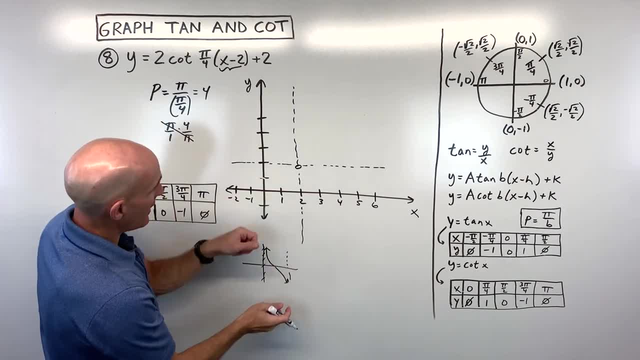 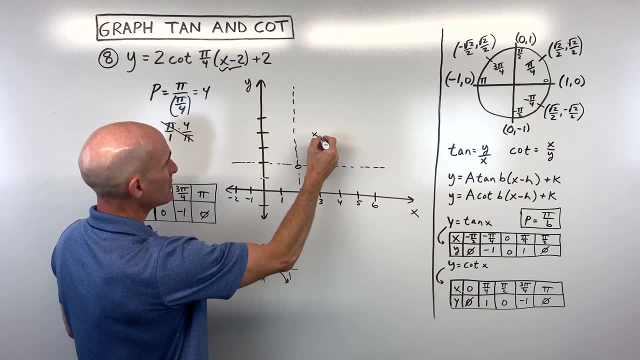 So in this case, what's going to happen is it's just going to be stretched by a factor of two. So what we're going to do is we're going to have a vertical asymptote here. This next step over, we're going to start at two up. 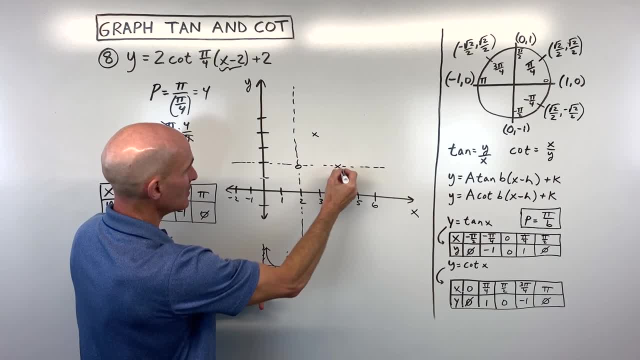 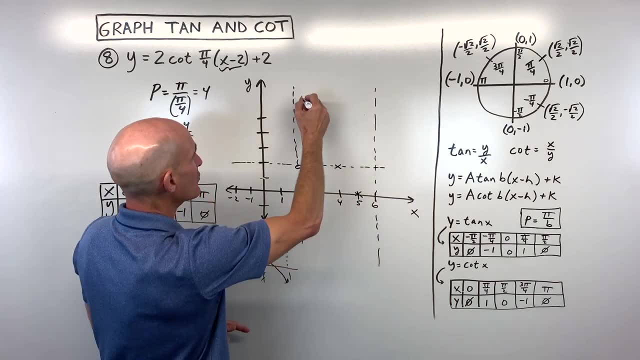 OK, then we're going to go back to the x-axis right here, which is going to be here, And then we're going to go two down And then we're going to have our other vertical asymptote right like so. OK, and so there is our basic cotangent graph. 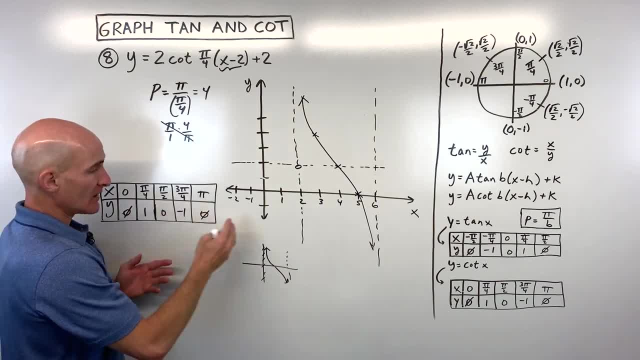 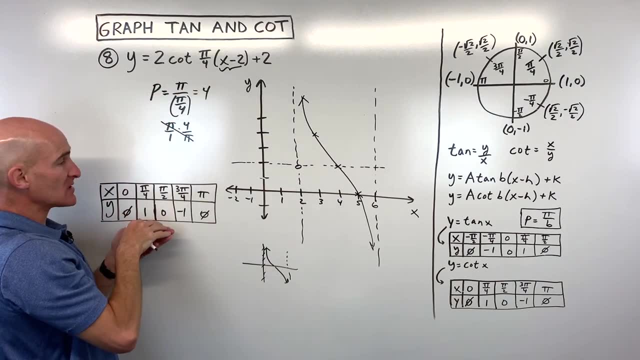 And you got it. Now, if you want to use the table method again, you want to memorize these values, or you can get it from your unit circle. Let's go through our transformation. So the a value two is multiplying all the y values by two. 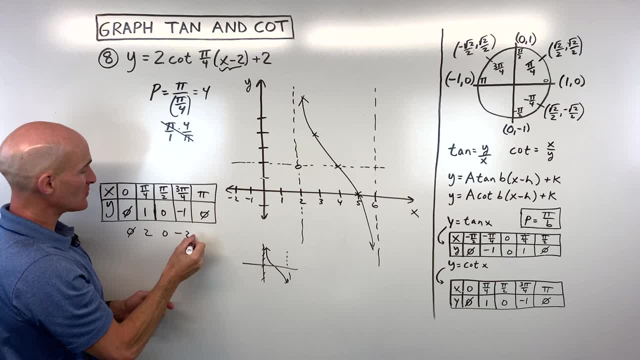 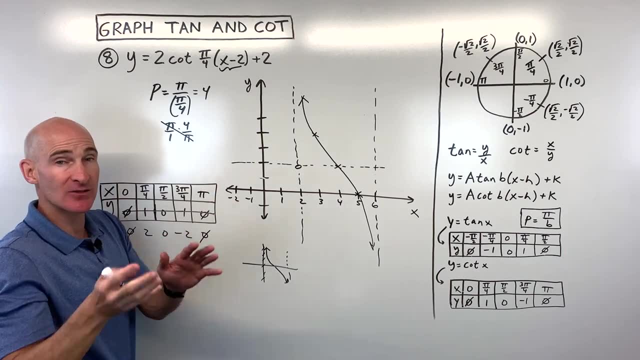 That's a vertical stretch. So I'm going to multiply all these y values by two, cross off the old ones. The pi over four is going to affect the horizontal direction x values, but it has the reciprocal effect. So I'm going to multiply everything by four over pi, all the x values. 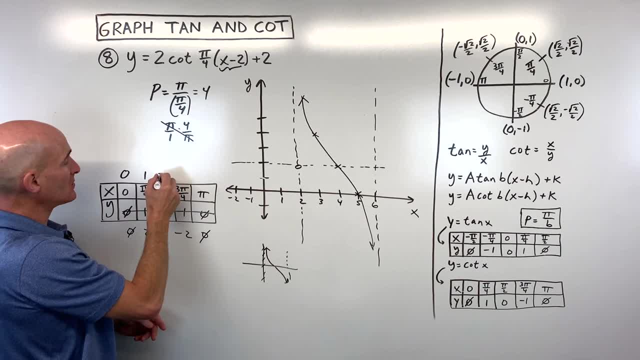 So that's going to give me four over pi. That's going to give me one, two, three and four. Cross off the old x values. The minus two is going to shift the graph right two. So I'm going to add two to all these x values.